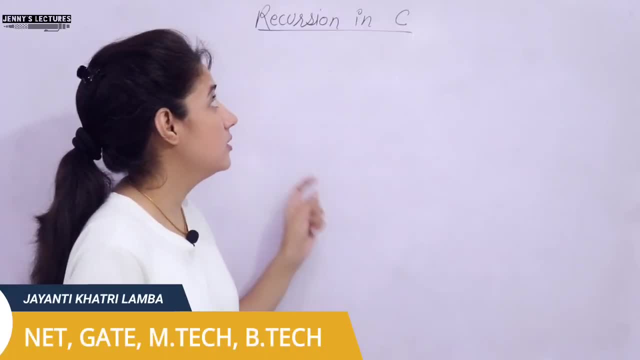 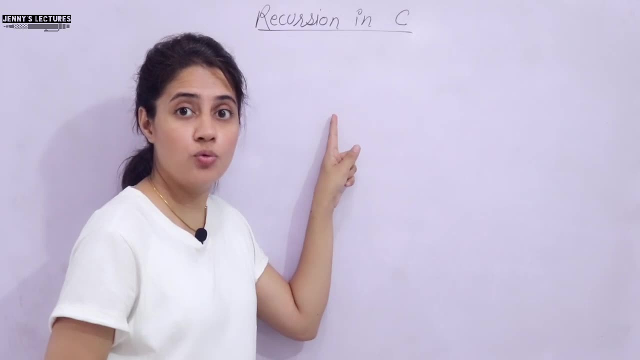 So in the series of learning C programming from this video, I am going to start recursion in C. This is very important topic in C and generally in gate exam. you know you find questions on recursion right and during interview also they used to ask question from this topic and you can. 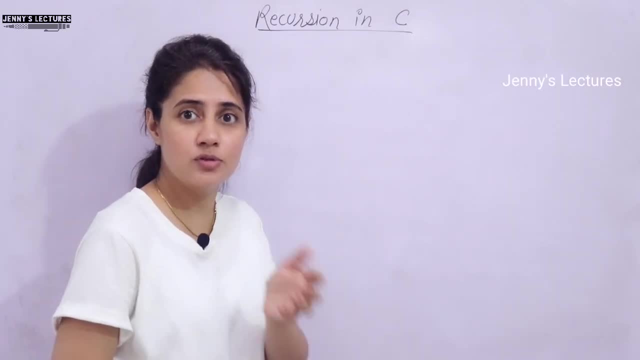 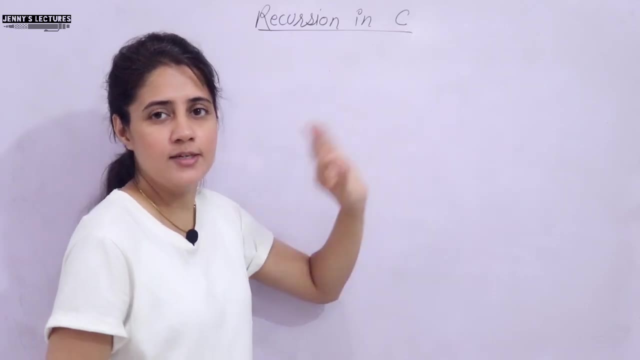 say it's a little bit tricky, or you can say tough for the beginners, for the students who are, you know, beginners in programming language, who are beginners in C language, they'll find this topic very tough. but it's not like that. If you got what is recursion, the basics and how you are going. 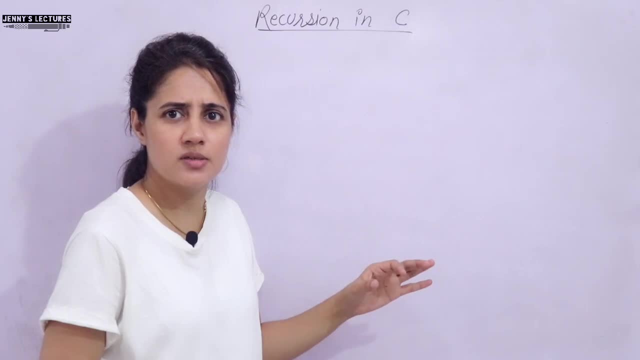 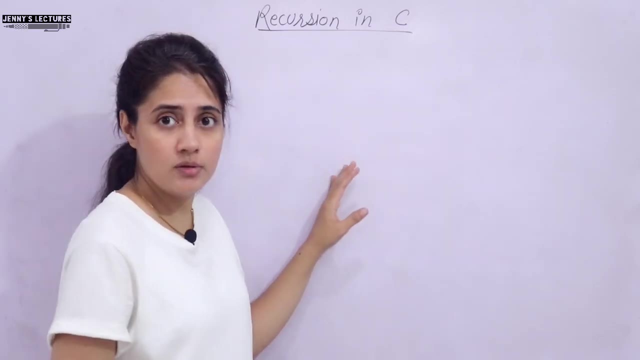 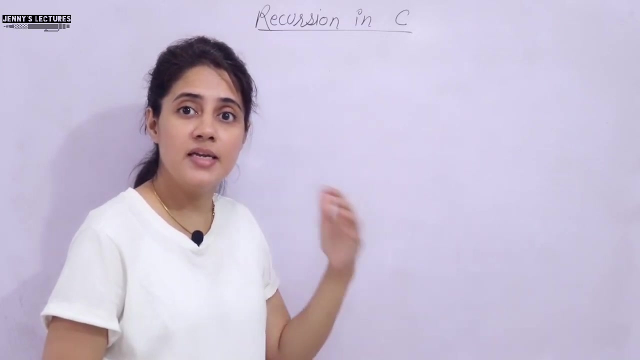 to solve the programs which are using recursion- the process. you will definitely say that it's not that tough, right? So we'll discuss everything about recursion in this video. we'll see what is recursion and we'll see a simple program using recursion, right? but there are many things about. 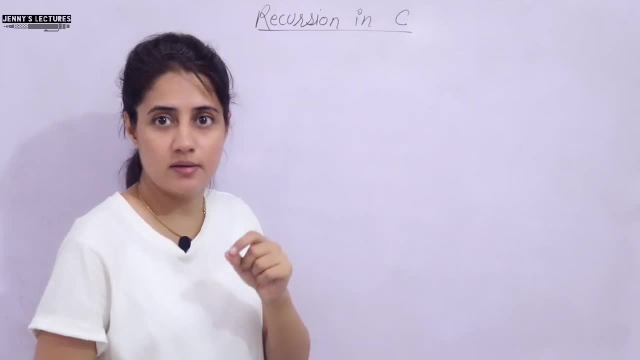 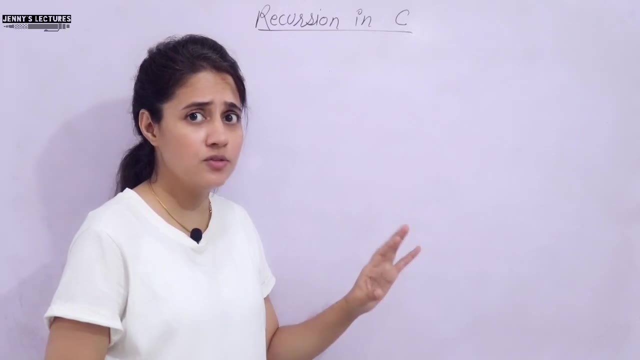 recursion, like types of recursion, direct and indirect, tailed and you know known tailed adversarial. So we'll see what is recursion and we'll see a simple program using recursion right, advantages of recursion, drawbacks of recursion, why we use recursion and some problems, also everything we will discuss recursion from the basics right one by one in later videos. 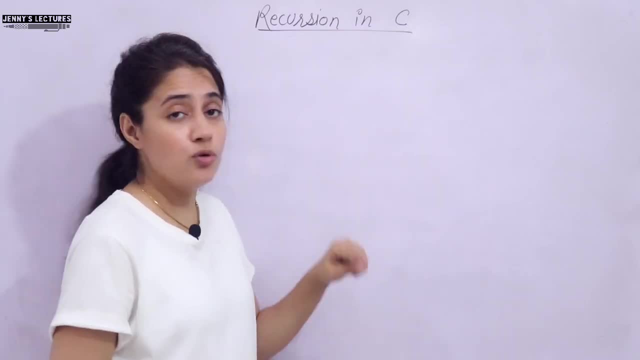 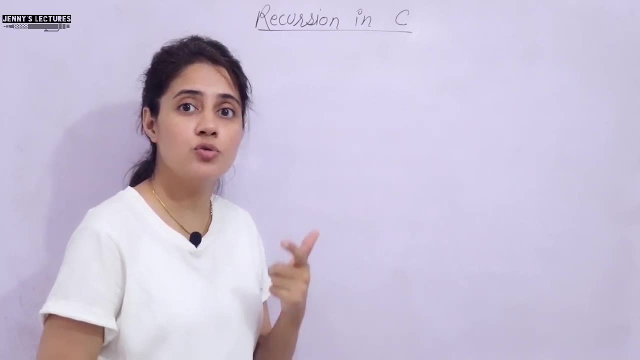 So this video is like introduction to recursion, right. but before that, just want to tell you one thing: if you are preparing for gate 2023 exam or will be preparing for gate exam, then an academy is going to start a batch RO1 for gate and ESC from 13th of October. In this course, the top 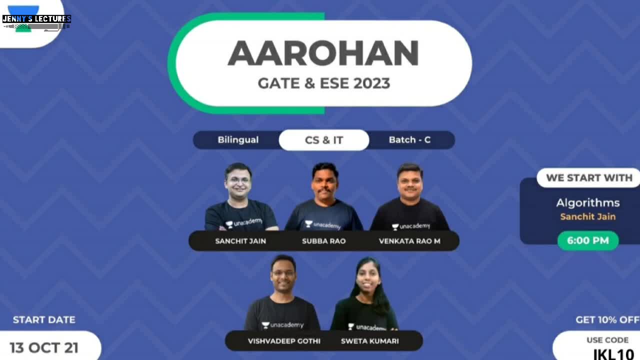 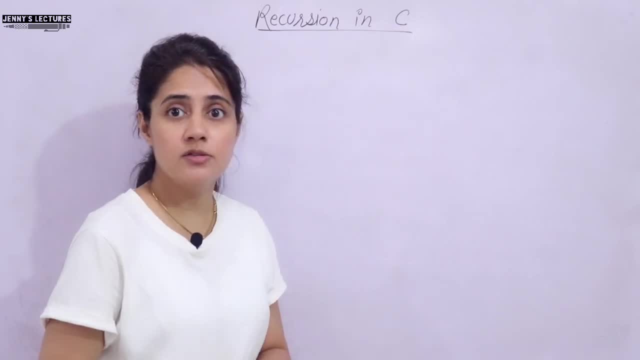 educators will be covering all the subjects of CS and IT, which will help you to prepare for the gate exam. This course includes preparation strategies, some tips and tricks, practice questions, numericals, along with the detailed explanation of the concepts. and you know this course will be covered in both Hindi and English, but notes will be given to you in English only. 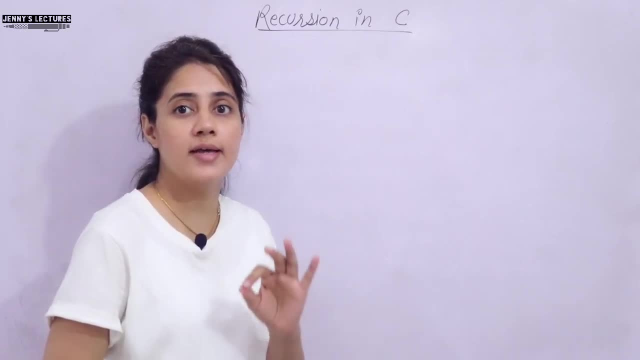 and you can. you all your doubts will be clarified in the doubt clearing sessions in the course, right. but this one is paid. but if you will use my code JKL10, then you will get extra 10% discount on your paid subscription. One more thing: they are also going to conduct a combat. 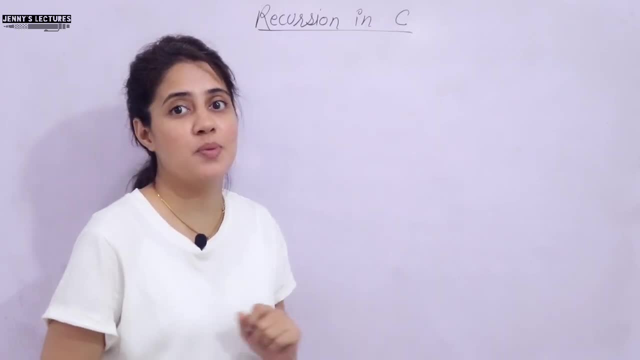 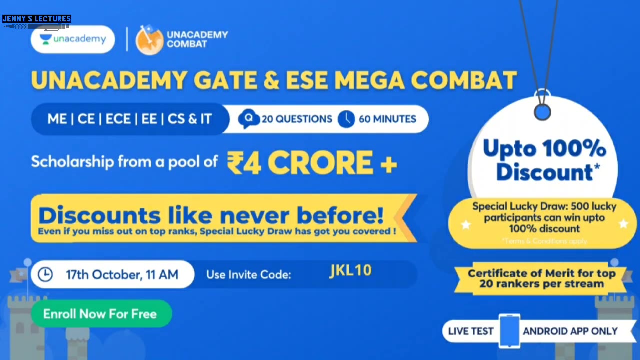 it's like the ultimate scholarship test for gate and ESC aspirants, which would be on 17th of October. So in this contest you will get the original and challenging gate questions. you will get 20 questions and time limit would be 60 minutes. you can assess your preparation in just. 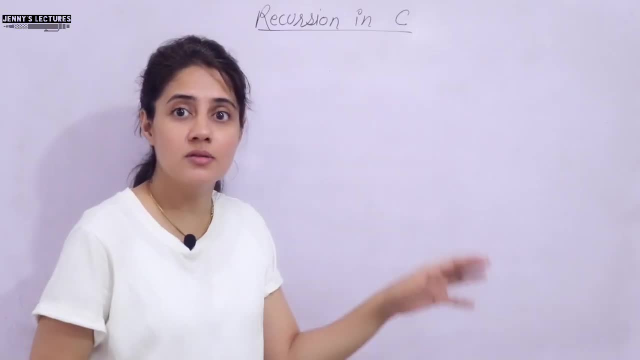 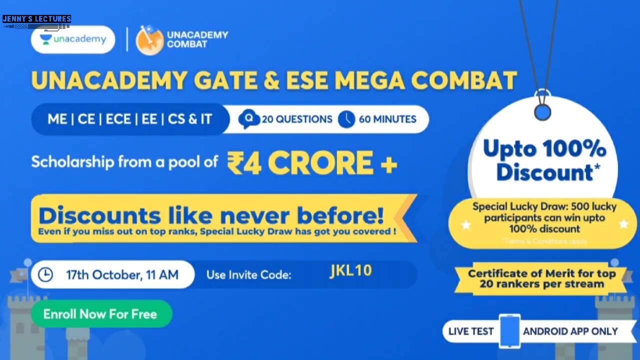 60 minutes and you can also see where you are standing among the others using the live leader board. that would be updated after every question and if you take it live, you will also get a chance to win some exciting awards. the detail you can see on my screen and you can take it live. and you can. 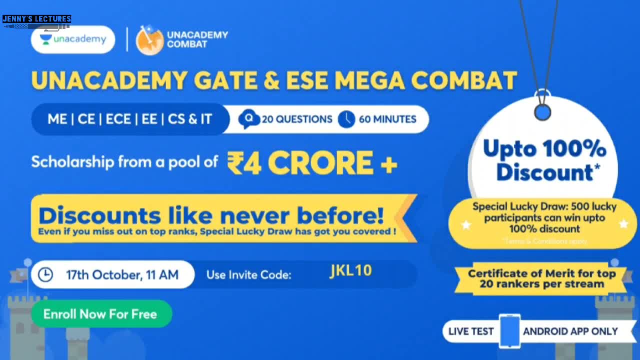 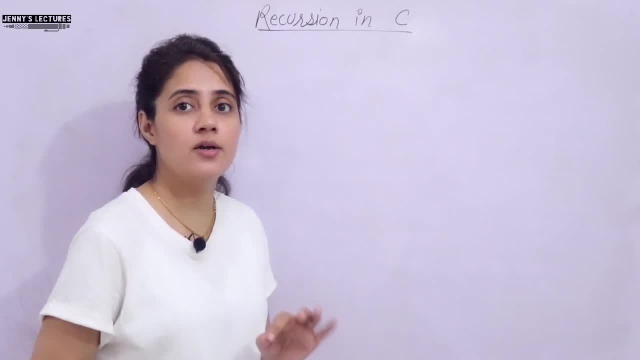 take this test for free. you just have to enroll the enrollment link I'll put in the description box of this video. you just have to go to that link, scroll down, pick up the right test for you and just click enroll and use my code JKL10 to unlock the test. and there is one more great offer. 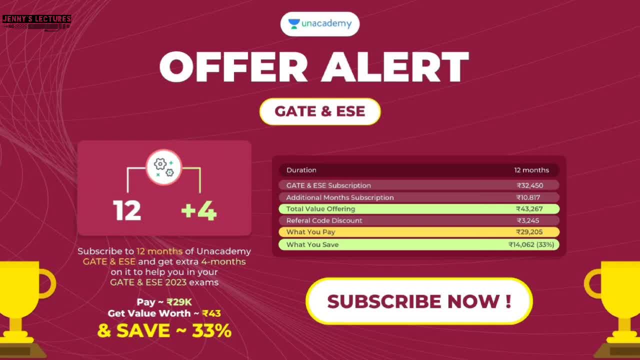 for you on unacademy, if you subscribe to 12 months of unacademy gate or ESC plan, then you will get extra four months. means you just have to pay for 12 months and you will get 12 plus four months for your preparation. you can see the detail of the price on my screen. so all the relevant links. 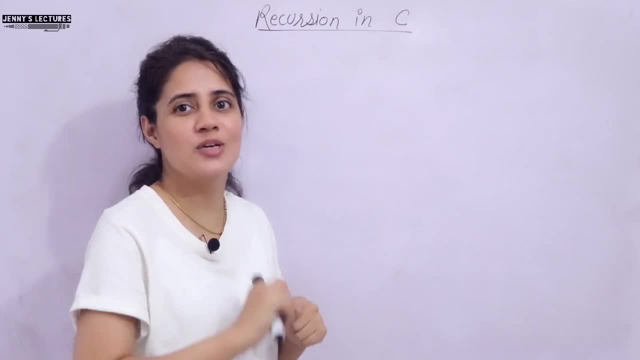 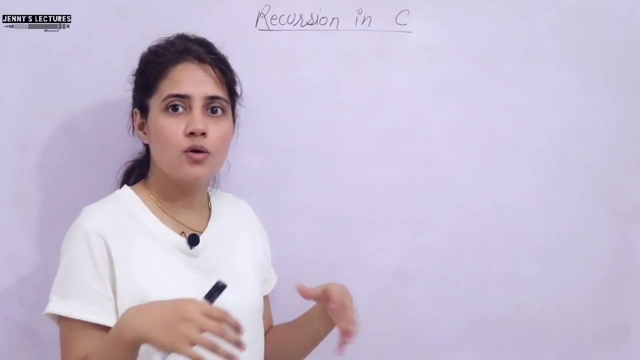 and the code I'll put in the description box of this video. if you are interested, you can go and check out. now let's discuss what is recursion in C first of all. what is recursion? it's simple: when a function call itself, then it is called recursion. see, we have discussed like this is. 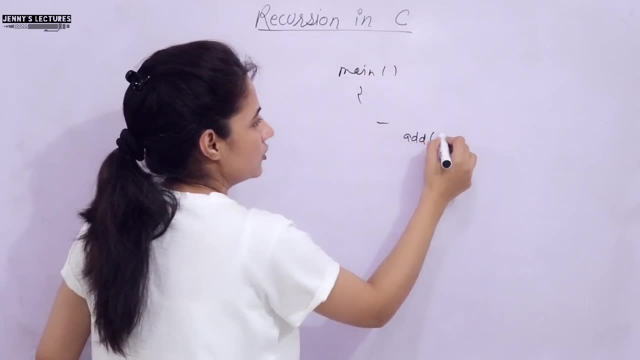 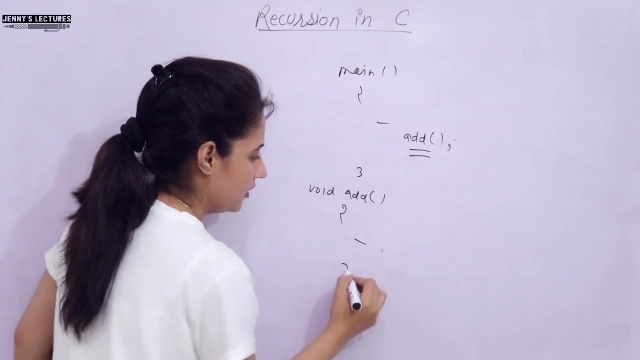 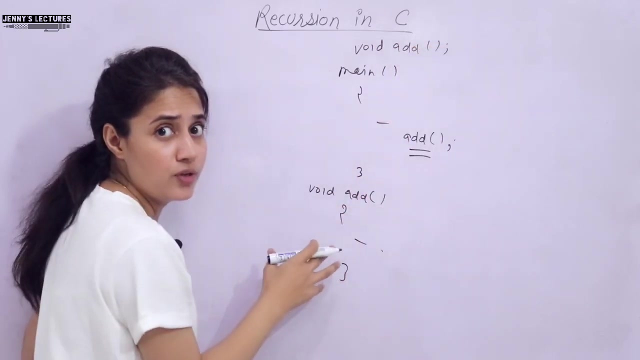 main function and here we are calling a function, suppose add. we have one function, add, we are calling this function here, right, and here we have, suppose you know, add and the definition of this function. we have prototype, like void, add something, this kind of thing. so this is what function. 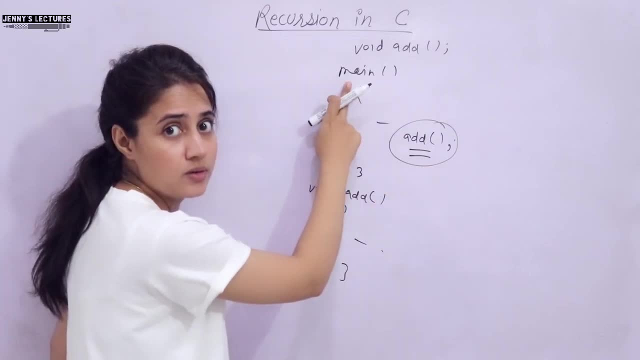 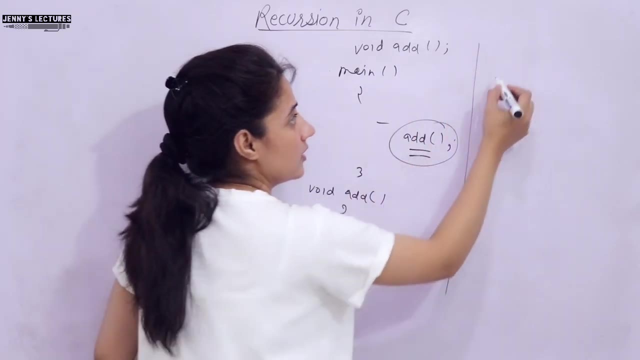 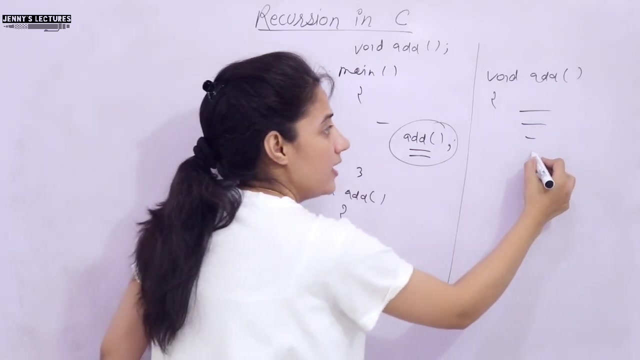 calling this function. we are calling in main function, right? so this is what calling function, this is what cold function. but but if I write something like this, I'm writing void add. this is I'm writing, suppose, definition of the function. here I'm writing some code and in this function 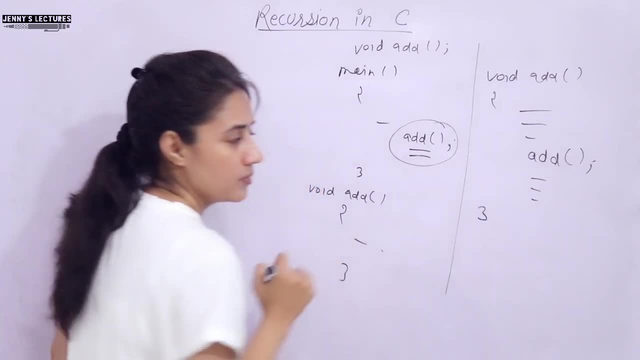 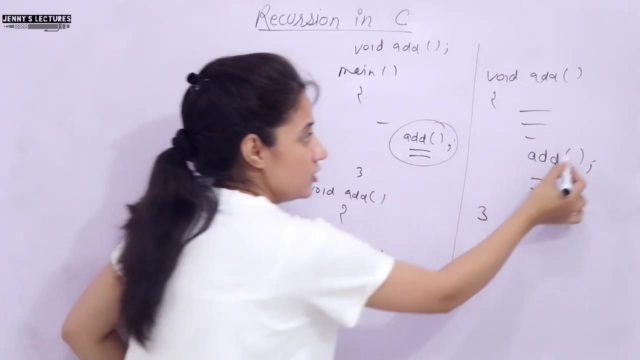 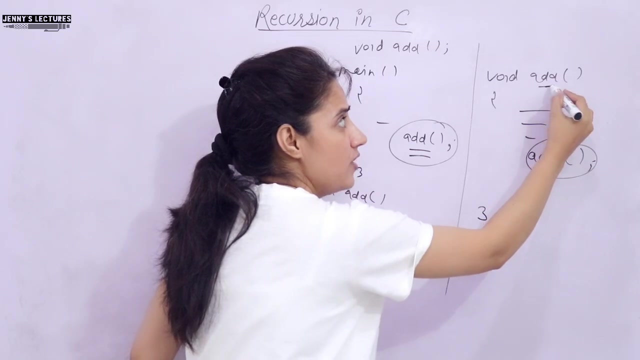 itself. here also I'm writing some code: function calling. I hope you know the syntax of, you remember the syntax of function calling. so this is what function calling and where we are calling this function. add the same, the same function. so the same function is calling itself means this function is calling itself, this process. 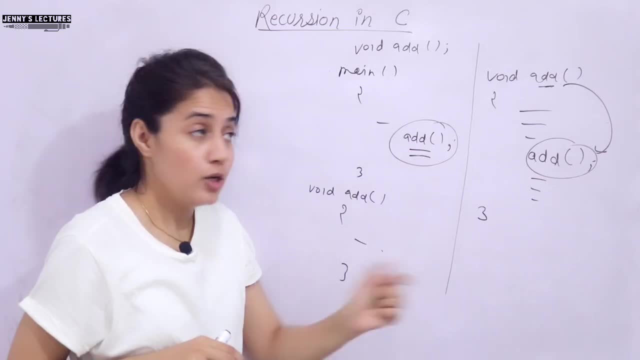 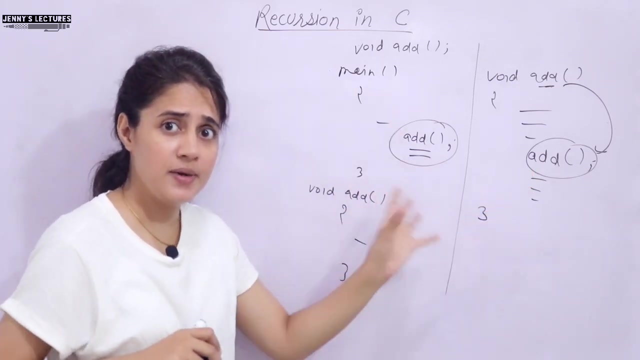 is called recursion, right, and this the function can call itself directly or indirectly. that is why types of recursion comes: direct recursion, indirect recursion, tailed recursion, non-tailed recursion- that we'll discuss in next video. right, this is like simple introduction to recursion. so recursion is what? when a function call. 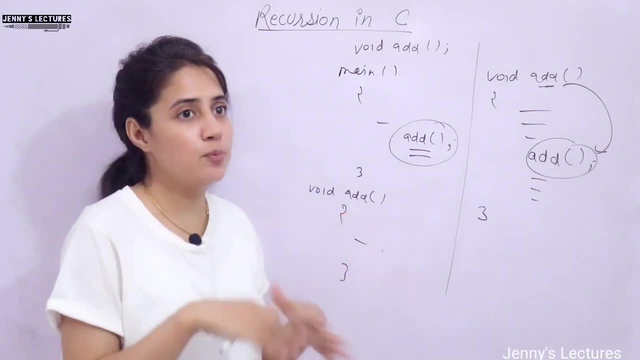 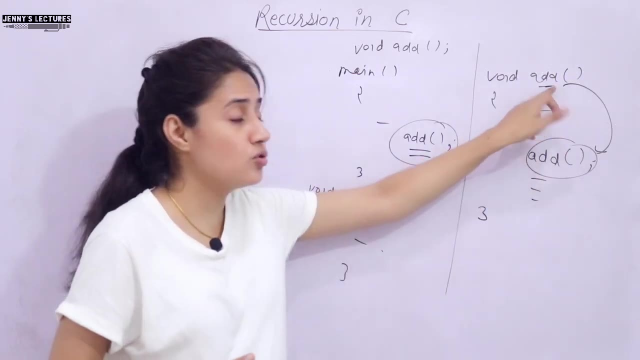 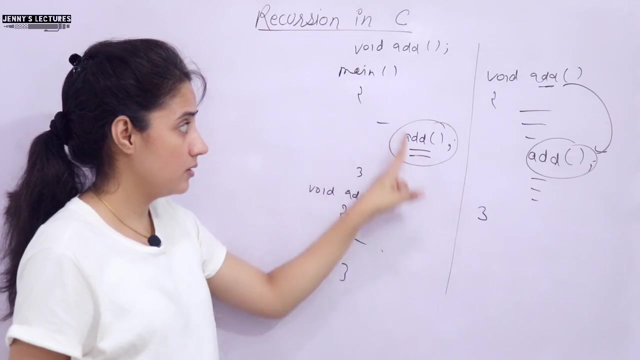 itself, directly or indirectly. that thing is called recursion, that process is called recursion. that's it. and this, this function is called recursive function. the function which is calling itself, this function is called recursive function. that's it. I hope you got the difference now. here we are calling in main this function, but here this function is calling itself. so this is called. 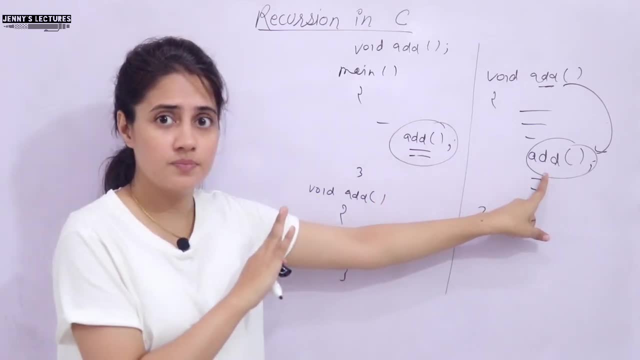 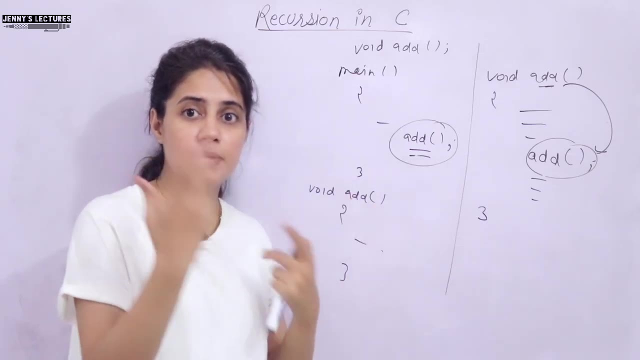 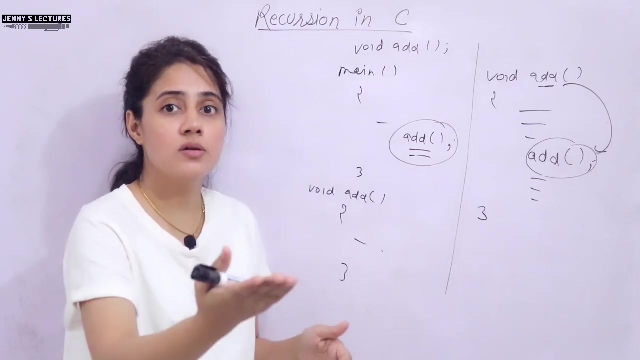 recursion. this is not recursion. this is simple function calling. this is recursion, right, like suppose? let's take a simple example. suppose in my class I have a student having name Rahul, so I'm calling Rahul like Rahul, but Rahul is not responding again, I'll call Rahul this time also. 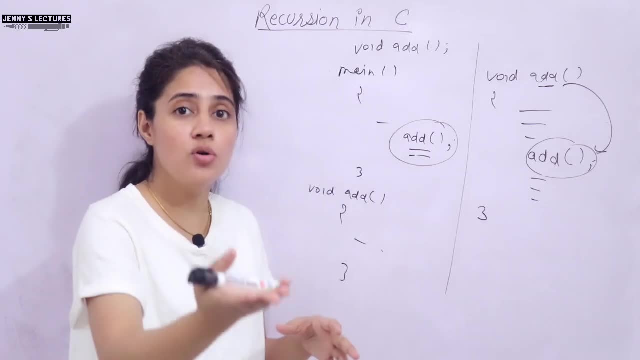 Rahul didn't listen and he's not responding. again. I call Rahul and this time Rahul responded: yes, ma'am. so now, like, suppose I'm one function, Rahul is another function, so I'm calling Rahul and when Rahul will respond, just stop. that's it right, but suppose I am calling. 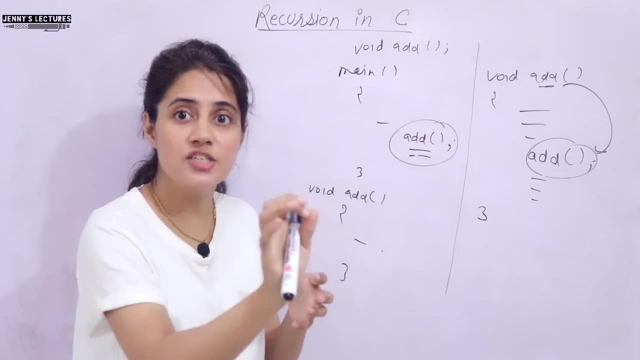 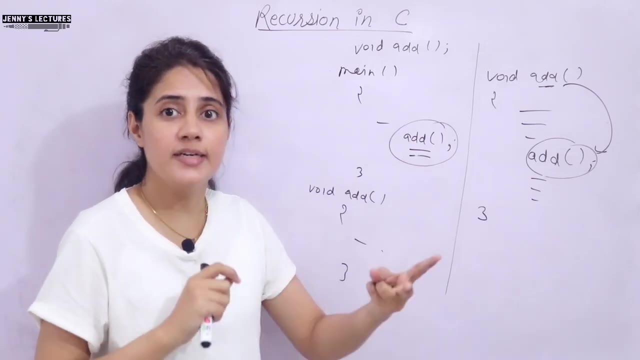 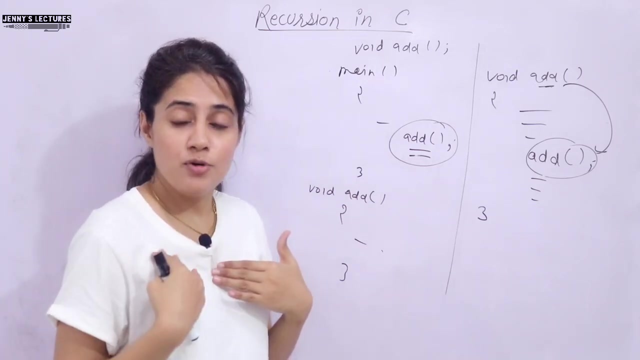 myself. so in the previous case the termination condition was: when Rahul will come to me I'll stop calling Rahul, right, and suppose I have called Rahul three times and after that Rahul came to me and I have stopped calling Rahul, but I am myself calling, like Jenny. I'm also Jenny, I'm Jenny and I'm calling Jenny itself, so I am Jenny only. so how? 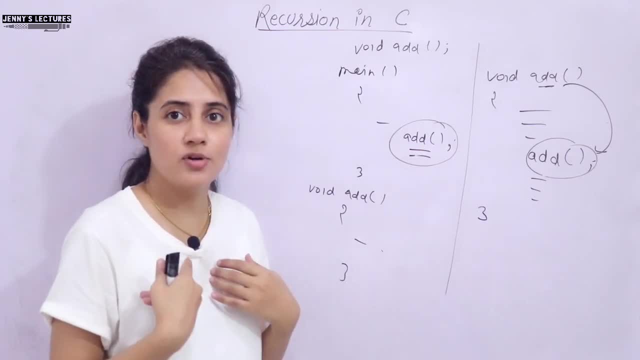 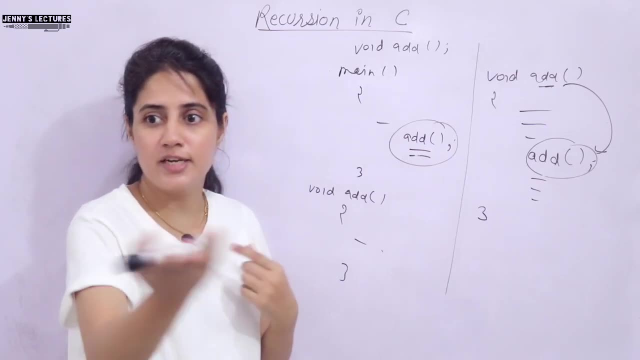 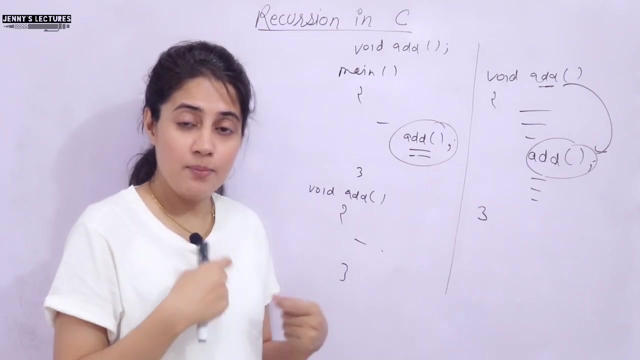 Jenny will come. like I'm calling Jenny, but I am Jenny only, so no how Jenny will come to me. so when I'm going to stop calling Jenny, I'm calling Jenny, Jenny, Jenny, but Jenny is not coming because I myself is no Jenny. so I myself calling, no, I'm calling myself. so this is what recursion. but now, 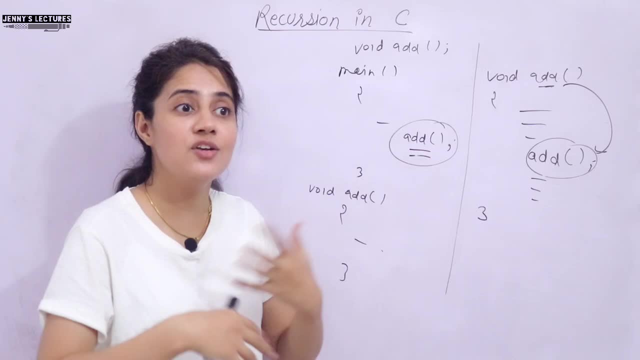 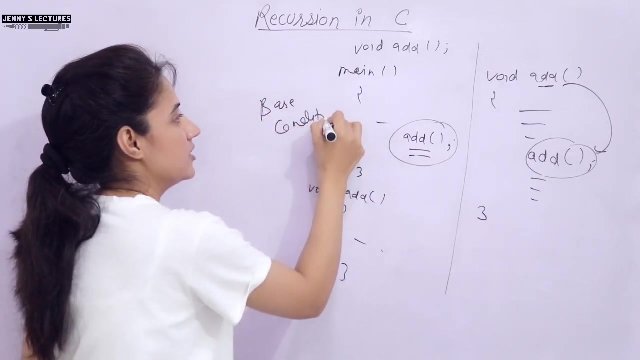 Jenny is not coming, so I'm calling Jenny, Jenny, Jenny. so this would be an infinite loop when I have to stop. so this thing is very important: when the recursion have to stop, the termination condition or the base condition in the recursion, this thing is very, very, very important. the base condition or the 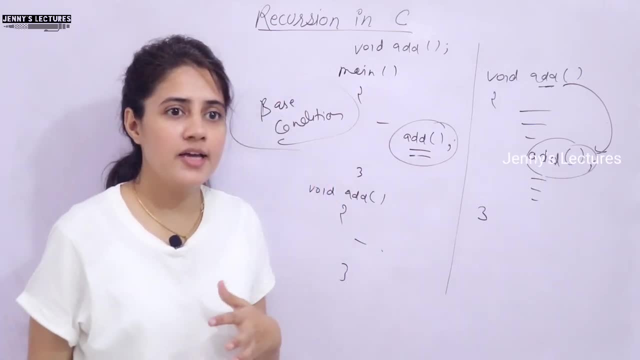 termination condition. so here I can, you know, put a condition like: after calling Jenny five times, I I'll stop. so I'll call Jenny five times: Jenny, Jenny, Jenny, Jenny, Jenny, and now I'll stop. so that is what the base condition when you have to stop the recursion. that is the base condition, that 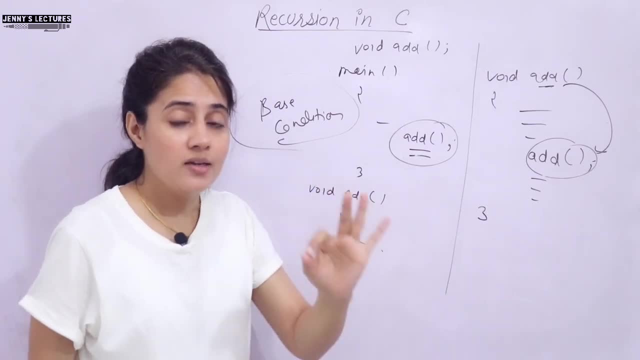 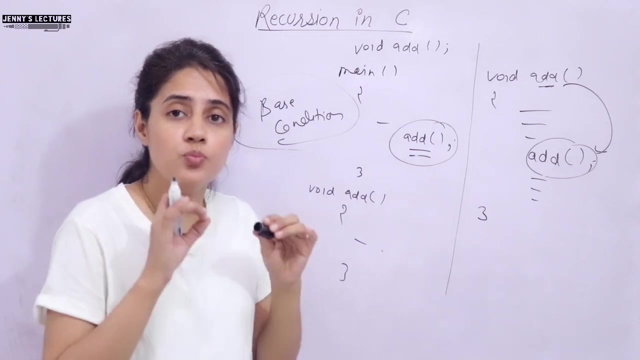 is the termination condition of recursion, and if you will not put that base condition properly then your program would be an in fine in infinite loop. maybe it will show some run time, you know, exception or infinite loop or undefined behavior it will show. so you have to put. 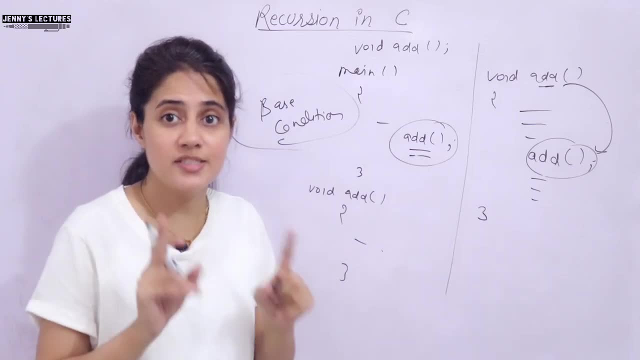 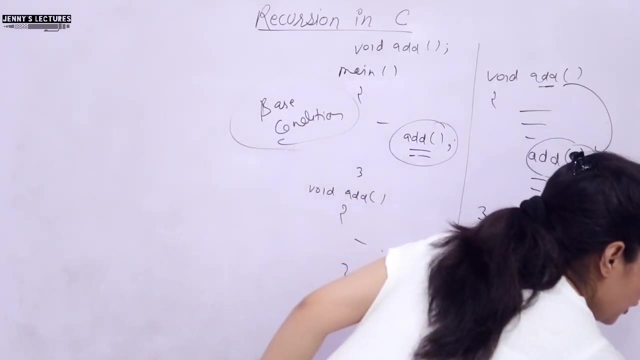 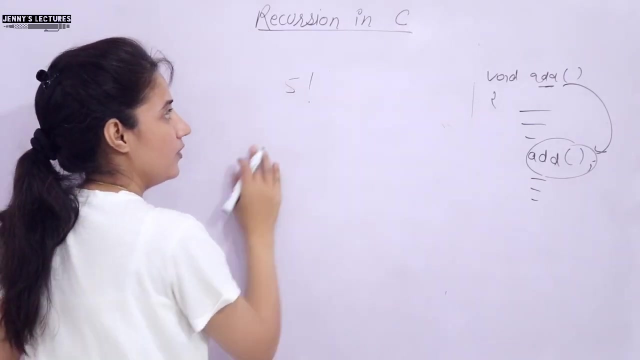 the base condition very, very, very carefully. this thing is very important when you are writing a using recursion. the base condition, See. let us take this example: if I am writing a program of you know finding factorial of a number, So I hope you know if I write 5 factorial. 5 factorial means 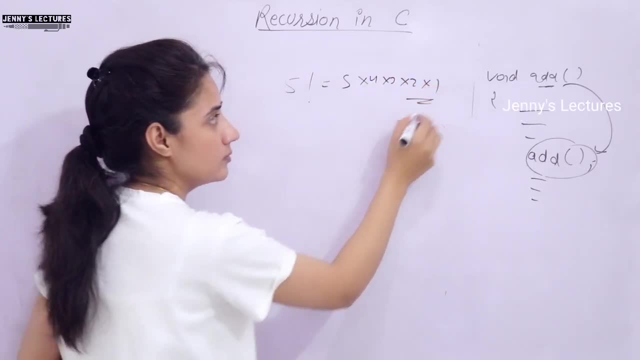 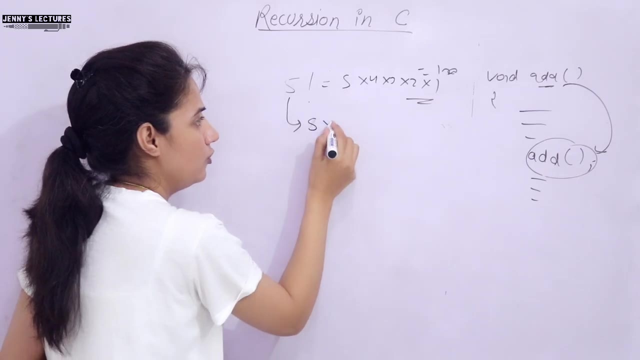 how to find: 5 into 4 into 3 into 2 into 1 is equal to 120, right? So 5 factorial. what I can write 5 into 4 factorial, that is also fine, right, 4 factorial. what you can write 4 into 3 factorial, that is also right. 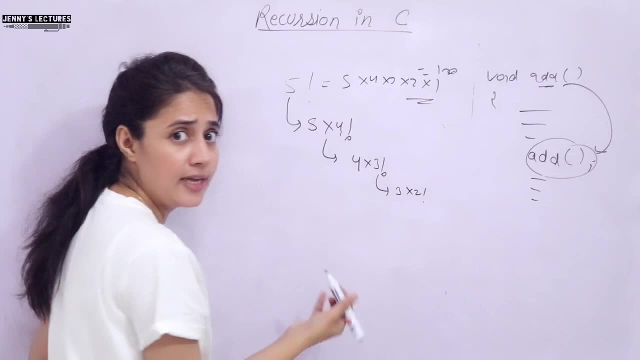 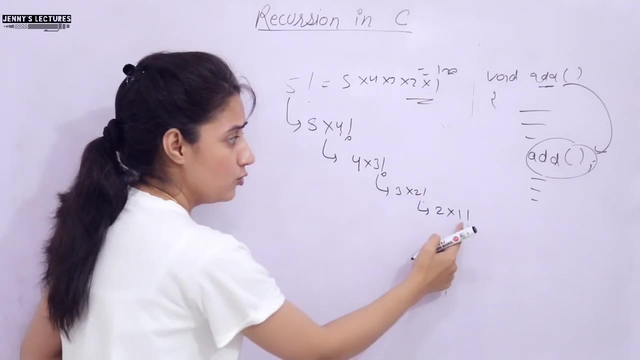 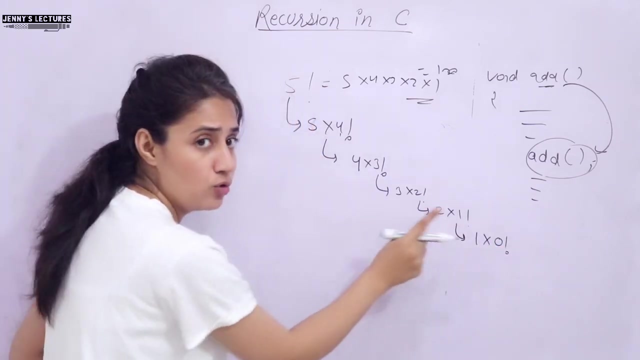 Again I can write 3 factorial. I can write 3 into 2 factorial. that is also right. 2 factorial. I can write 2 into 1 factorial. that is also right, right Now. 1 factorial is 1. or again I can write 1- 1 equal to sorry. 1 into 0 factorial. 1 factorial. you can write 1 into 0. 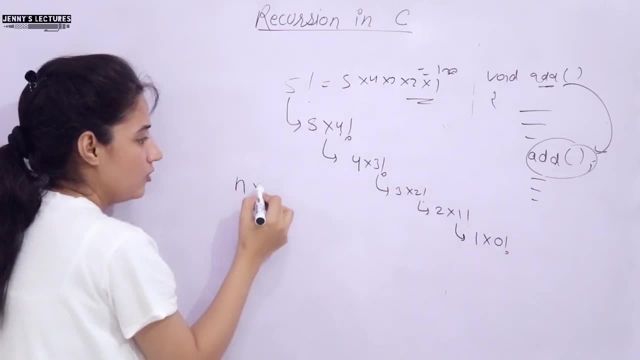 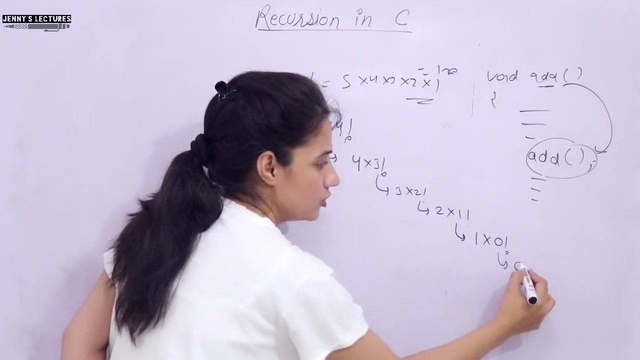 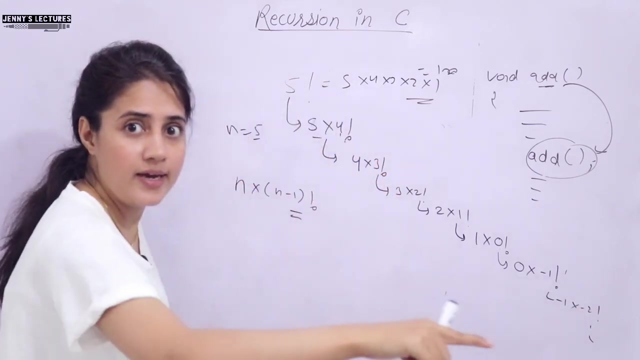 factorial right. So ultimately it means n into n minus 1 factorial Right. n is 5, so n into n minus 1 factorial. This is what I am doing, and again suppose. here I am again. 0 factorial means 0 into minus 1 factorial, then minus 1 into minus 2 factorial, and again. 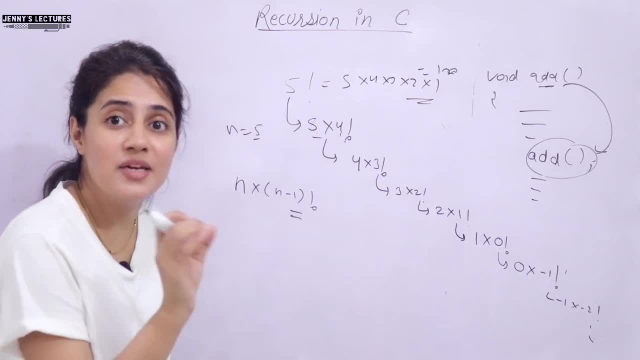 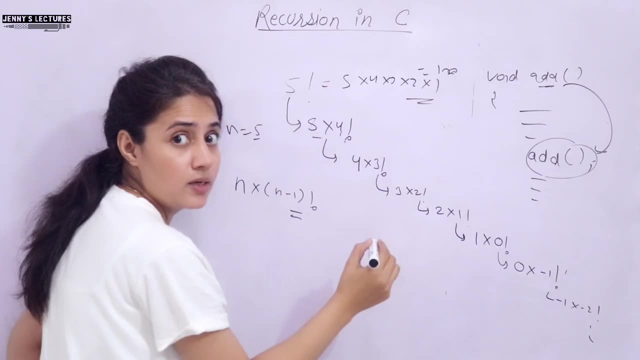 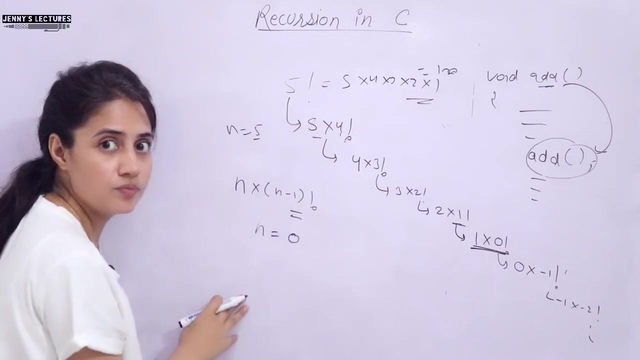 it is going on. If you will not put the termination condition, you have to identify where you have to stop, Where you are going to stop When, Here or here. also, you can stop When n becomes 0- right, because 0 factorial, we know it is 1.. 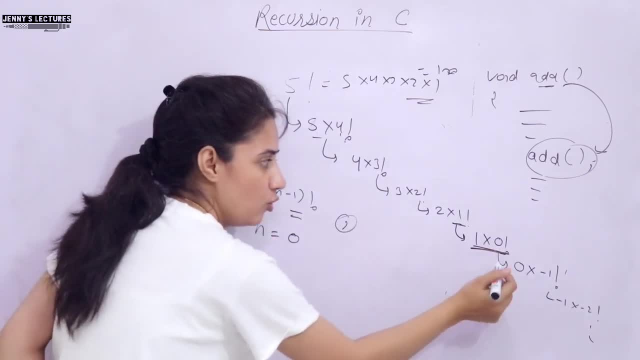 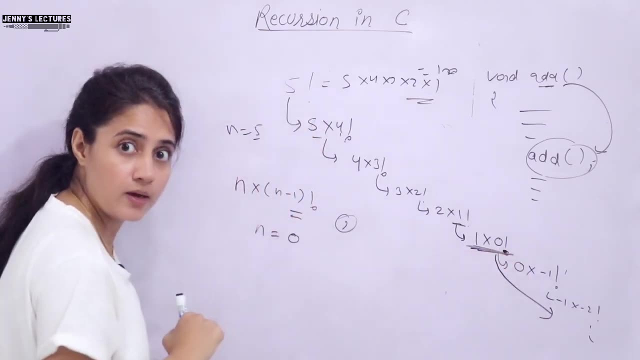 0 factorial means 1.. Now you have to stop. We will not move forward Further. we are not going to move here. we are going to stop right. or you can stop here like if n. you can also put this condition: if n is equal to is equal to 0.. 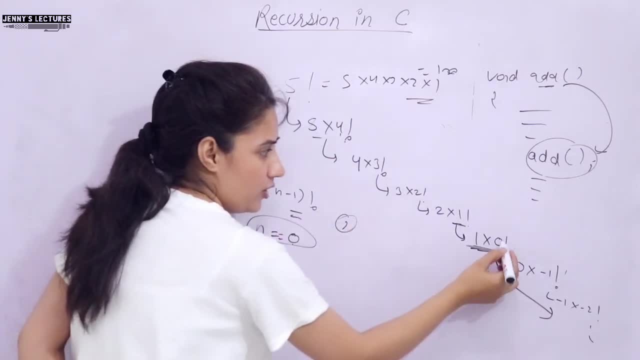 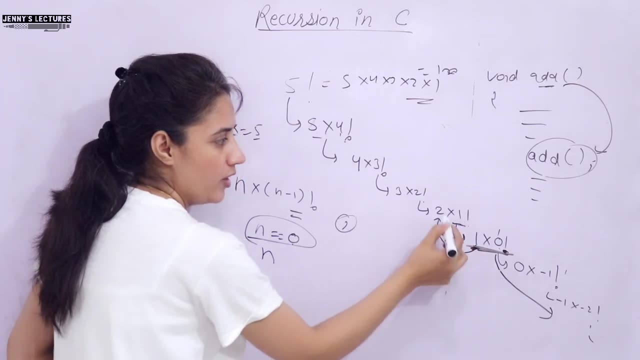 0 factorial means stop Now. 0 factorial means 1.. So from here, obviously, what we will do: we are going to return back. So we are. we are going to multiply this 1, then this 2, then this 3, then this 4, then. 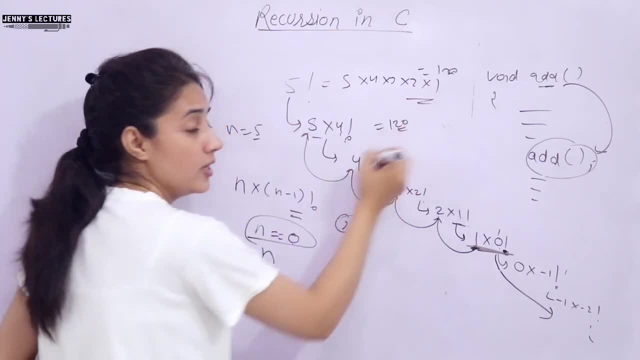 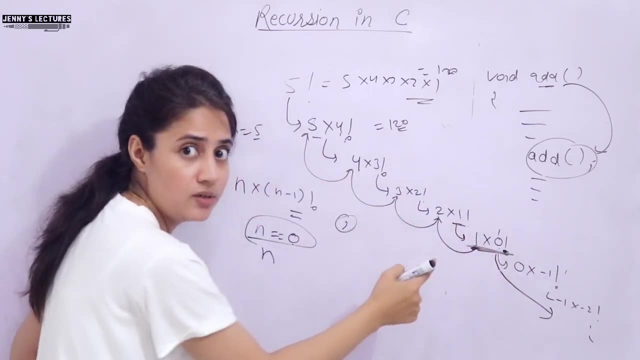 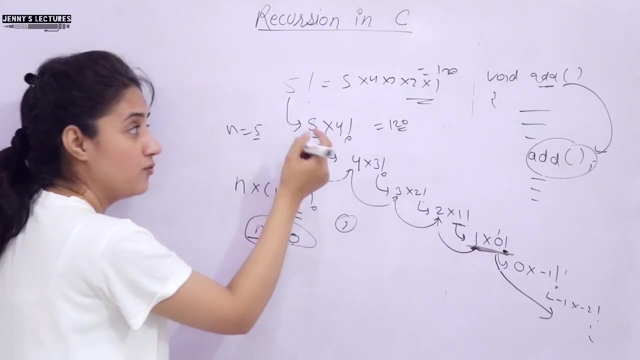 this 5 and ultimately you will get answer 120.. So we are moving forward as well, as, after finding the base condition, termination condition, in the same process we have to move backward, like this, like this: And from where you have started there you will have to stop now and after that you will get the. 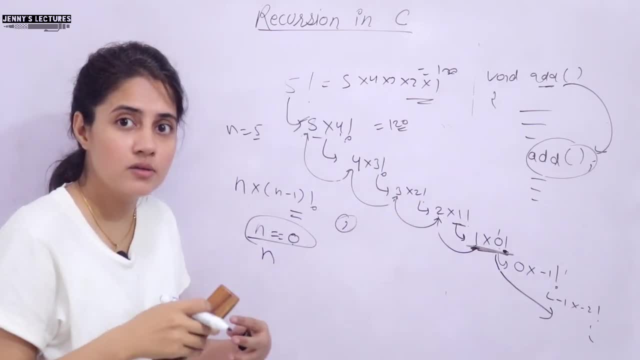 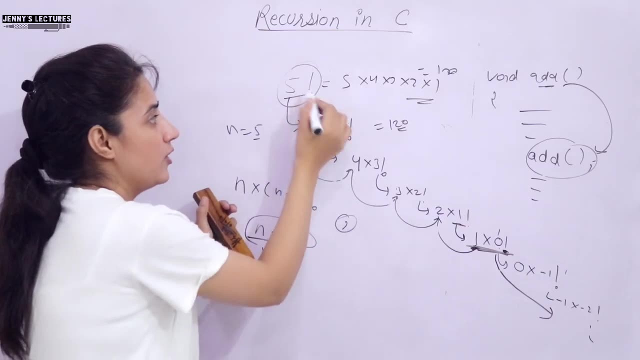 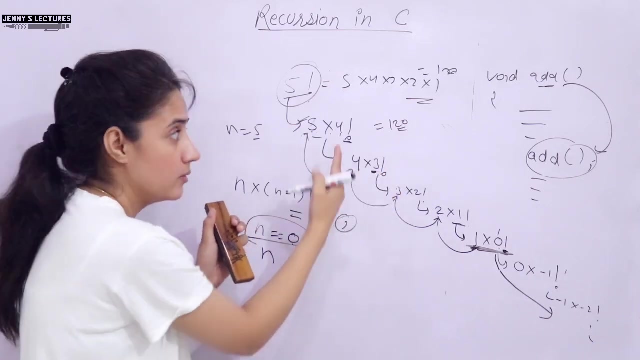 result. So what is the process behind the causal means? we are finally, you know you can say, dividing a problem into smaller one. We have divided this 5 factorial into 5, into 4 factorial. the smaller problem, The 4 factorial is 3 into 4, into 3 factorial. now the smaller one, because 4 factorial. 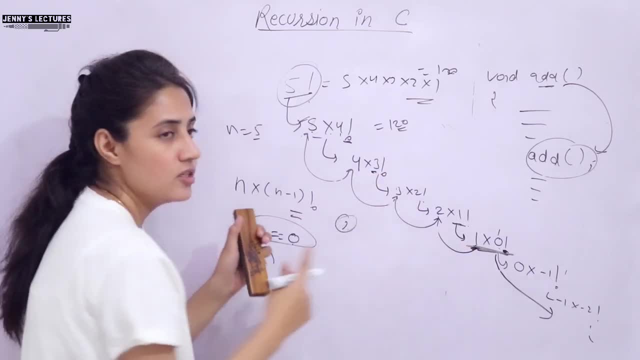 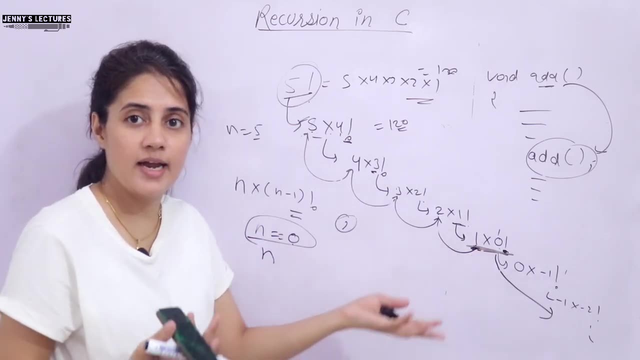 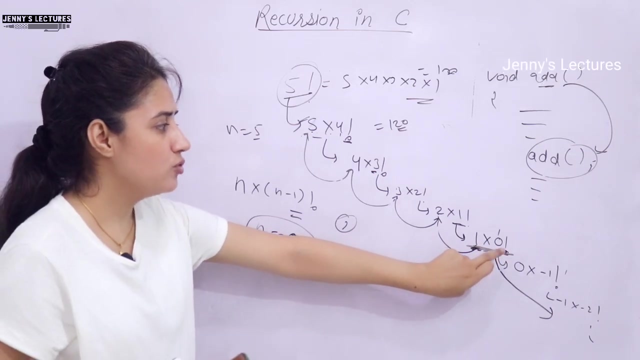 then 3, factorial. this is smaller one. Then again, we have divided this problem right And add some. we have added some base condition right, and that's it. That is what recursion right. So here, this thing is very important: where you have to stop, otherwise you will go forward and 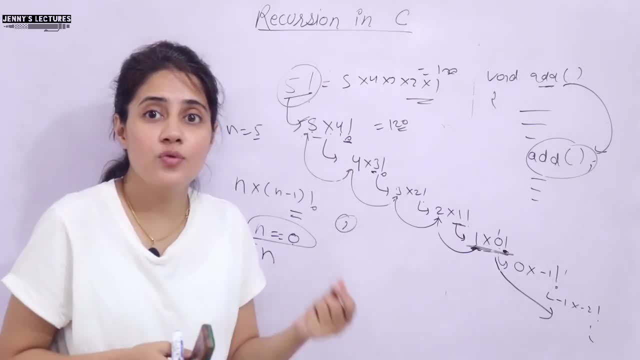 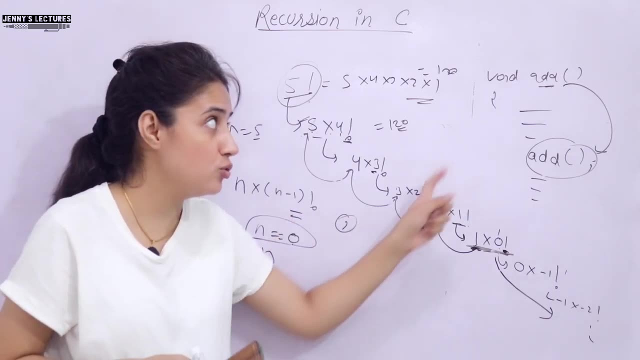 that would be an infinite loop. Maybe the stack overflow problem you will get Generally. you will get stack overflow problem when you are writing. you know programs using recursion- Because you don't put the right condition, the base condition, the termination condition, So you have to stop. 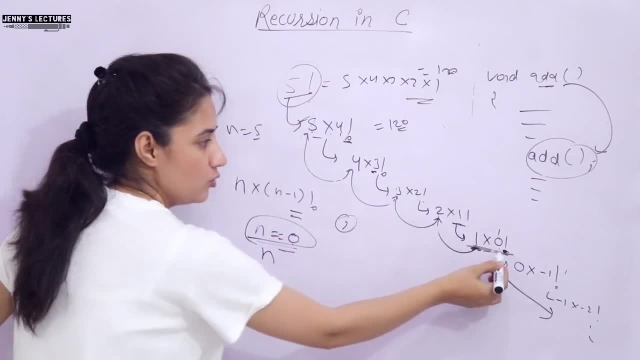 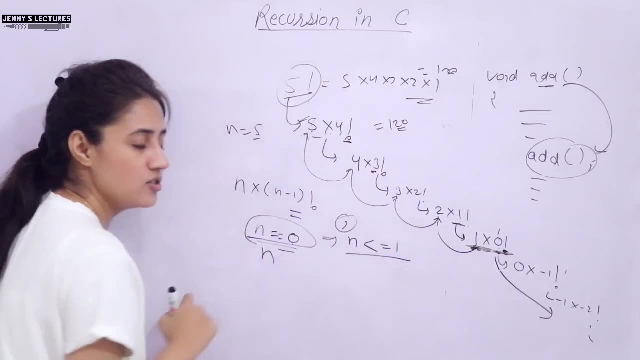 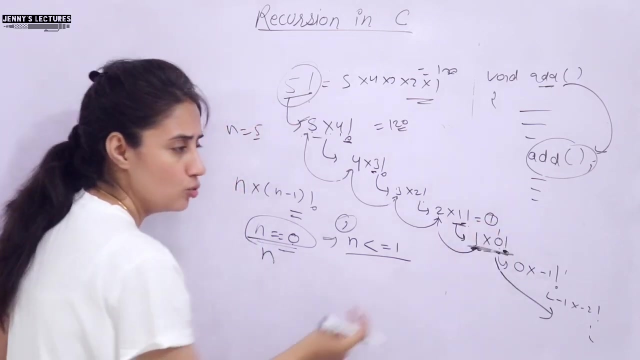 Here the termination function is: N is equal to, is equal to 0, you have to stop. or more precisely, I can say: if n becomes less than equal to 1, then stop. If n is 1, here also you can stop, because 1 factorial is also 1.. So no need to move further. 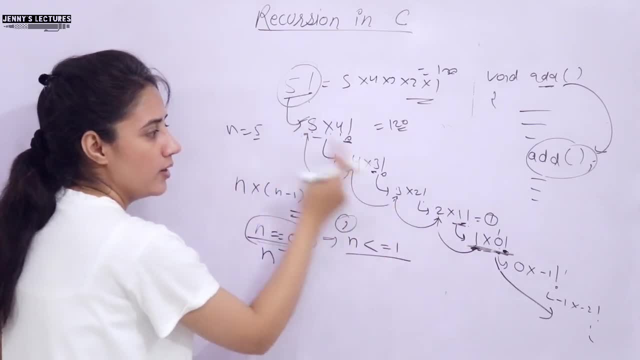 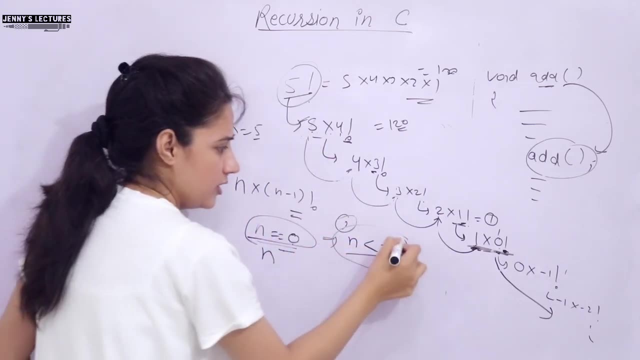 Here also you can stop and you can move backward, like you can multiply 2 into 3, into 4, into 5. That's it right. So that's it right, So that is you can say: this is the base condition. So here, if I put a condition, 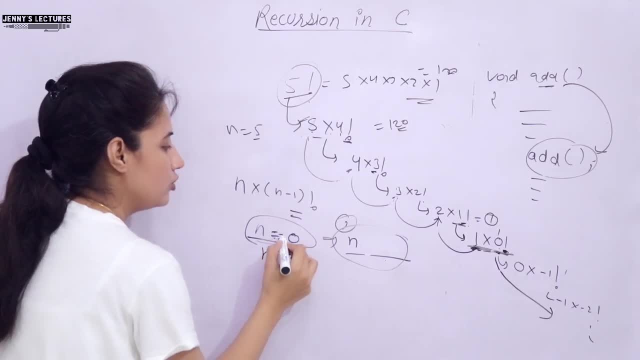 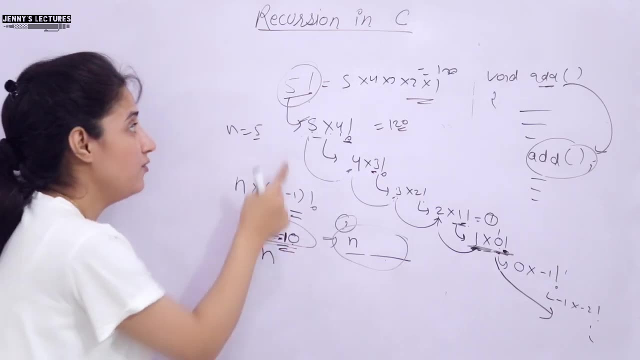 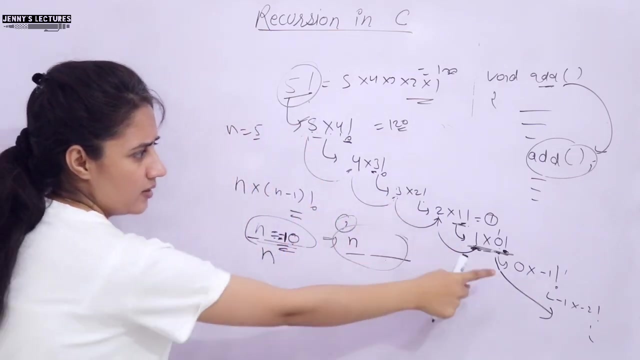 n is equal to is equal to 10,. the termination condition by default I have put: n is equal to is equal to 10, then you have to stop and I am finding factorial of 5.. So is there any chance of getting n is equal to 10 in this process? No, So ultimately you will move forward, forward. 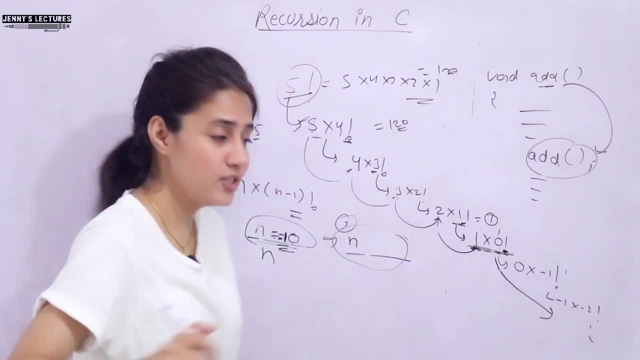 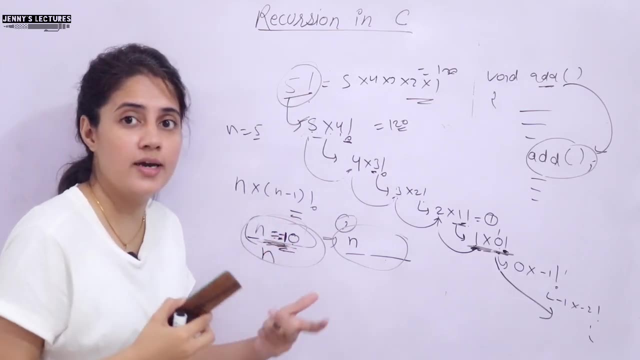 forward and this would be an infinite loop, This condition you will never reach to. this termination condition, right, And in this case you will find- you can find out the error, like stack overflow problem, Because every time you are going to call this function, the memory would. 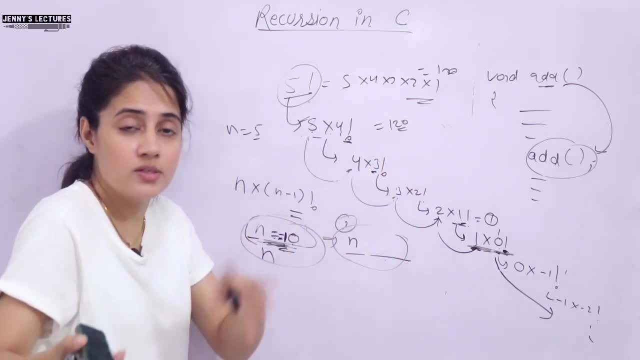 be allocated right And sometimes the memory would be exhausted. the stack memory would be exhausted, obviously out of you will, you know, run out of memory. So at that time you will find the error stack overflow problem right. So you have to find the error stack overflow problem. 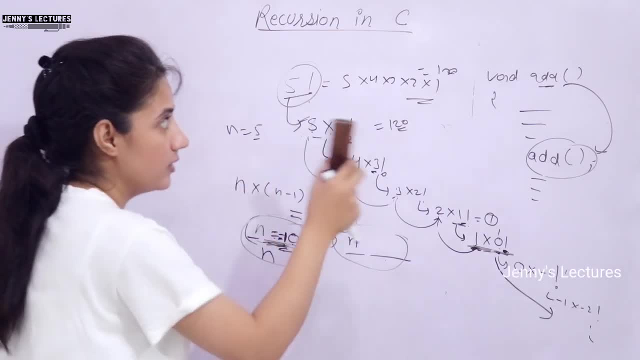 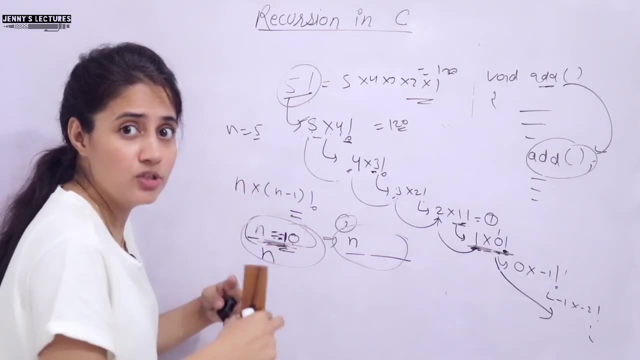 So how to put this termination condition very carefully in recursive programs. So I hope I guess you got the idea about recursion right. Basic idea: A function calling itself directly or indirectly. that thing is known as recursion in C, right? So let us take 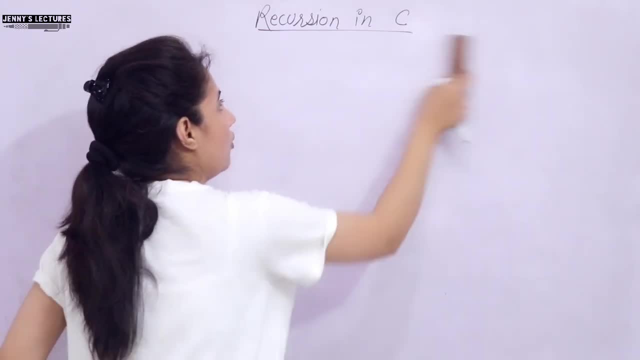 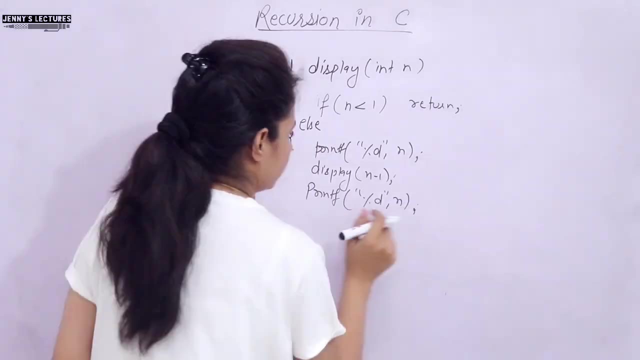 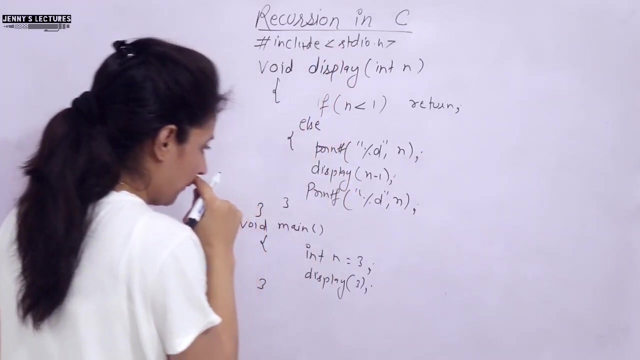 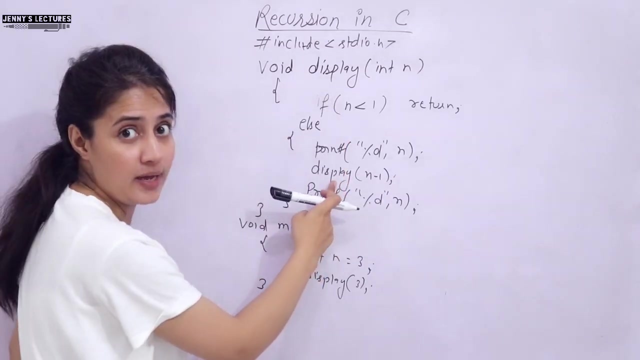 a simple example and we will see what kind of output you will get when you will run that program. so now, this is the- you know, simple program of recursion. why recursion? see, we are having a function, display, and in this function only i am calling display again. so this is what function. 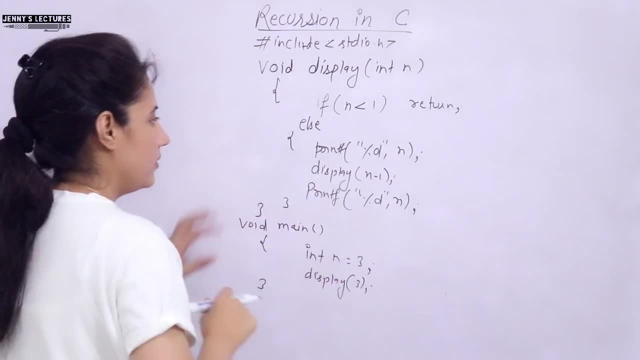 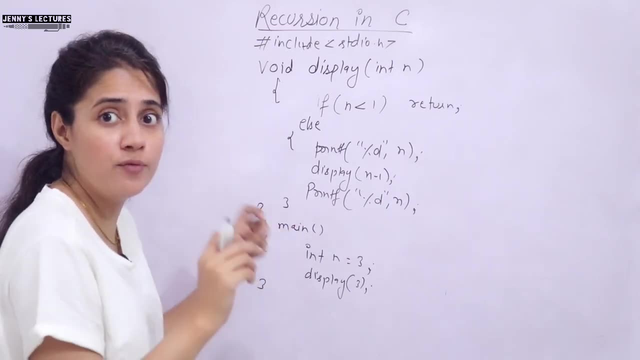 calling itself directly, right. so now how it will execute it, will it will be executed and what it will print. the process behind recursion. see, you have to follow the steps. only you have to understand this process very carefully. if you got the process of executing the program, having 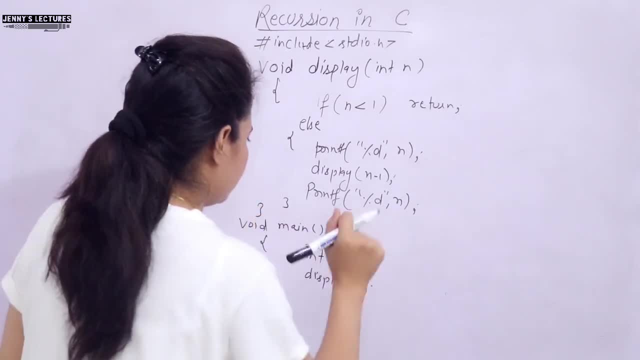 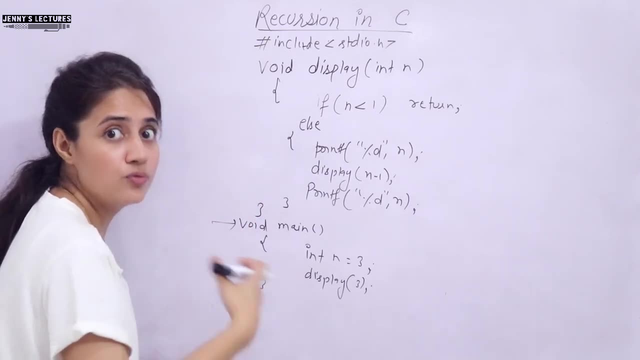 recursion. recursion would be like: it's very simple for you. so now, first of all, the control will go to the main function. so now, from the stack memory, one stack frame or activation record of that function would be. you know, hold in that memory. so one stack frame would be allocated to this main. 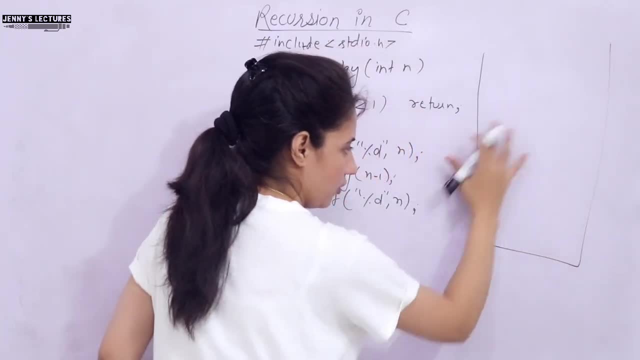 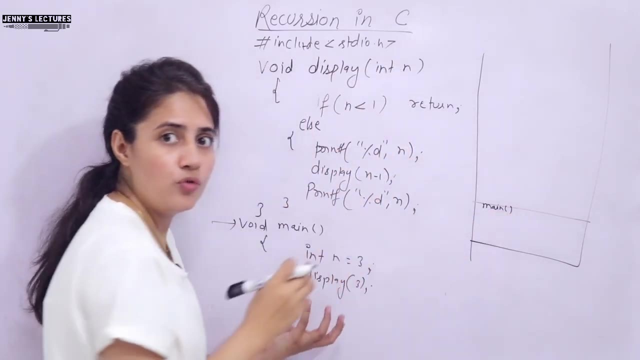 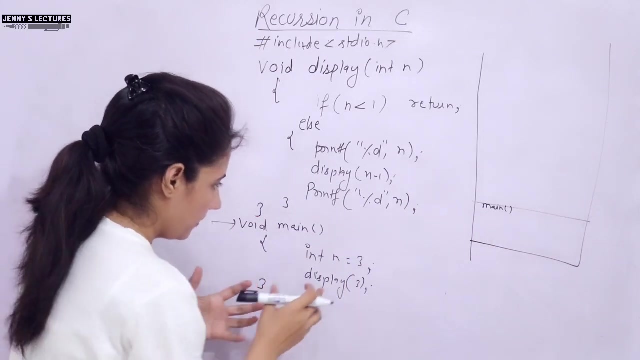 and let's say here, this is from the stack memory. here we have main, one frame for main. so here what would be stored, whatever the local variables here, you, you, you, that would be allocated here right now. here we have n is equal to 3, and many more things also. 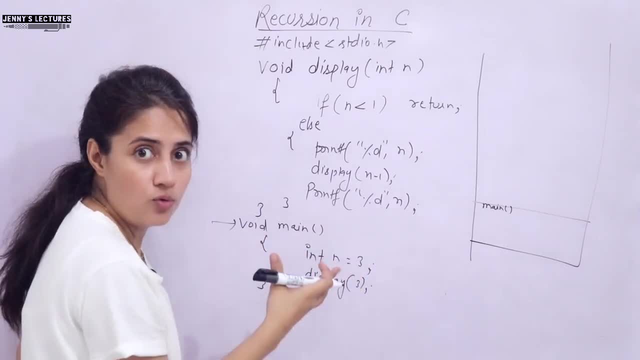 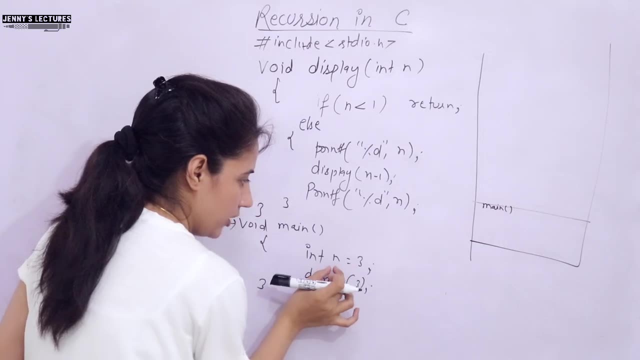 right, like you know from where this function has been called and what function it is calling, many things it is going to store, but here, for the simplicity purpose, i am just going to record here the local variable. so here we have n, so we have n, and n is equal to 3. so now next. 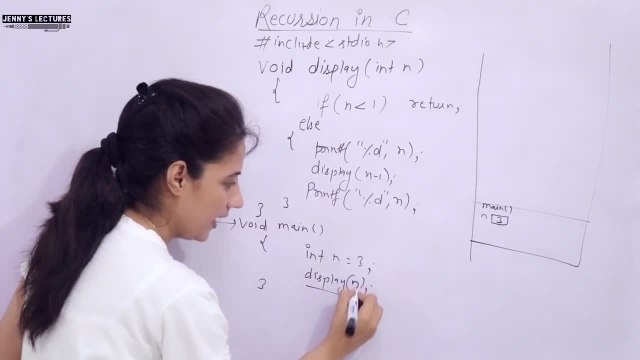 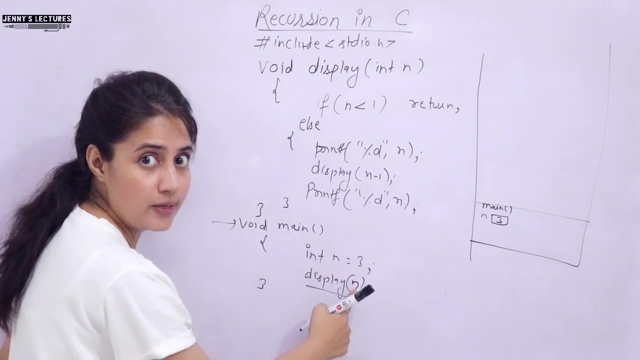 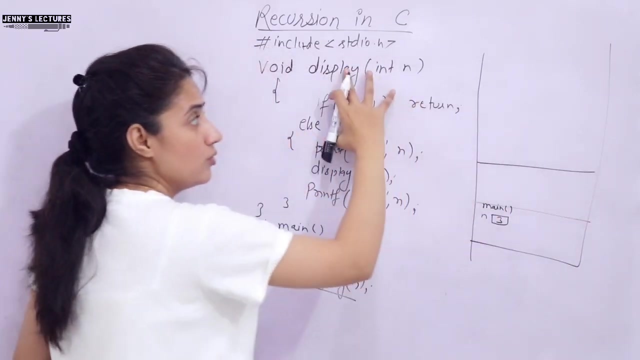 statement is display. we are calling, sorry, display n. obviously we are passing n. you can pass 3 also, but here our passing variable. so what value would be passed? 3, right, so now here, from here it is calling display. so means for display also, one frame would be allocated, the activation. 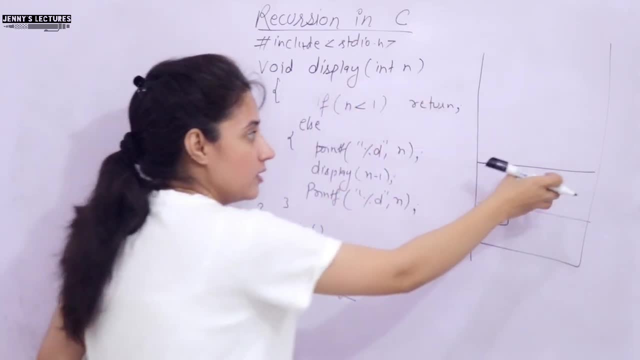 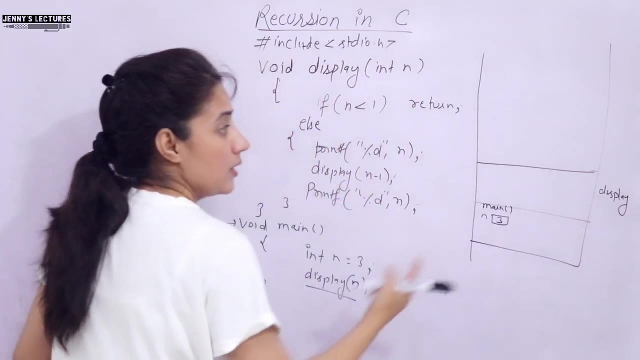 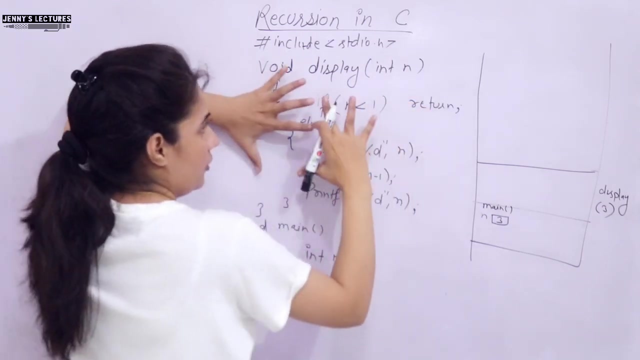 record for this display also would be stored here in the stack. some memory would be located, obviously, when you are going to call this function. so this is what for display, but here for display and three for display. three because anyway here we have n3, 3. So in this display function we have a local variable, the copy of these variables, you know. 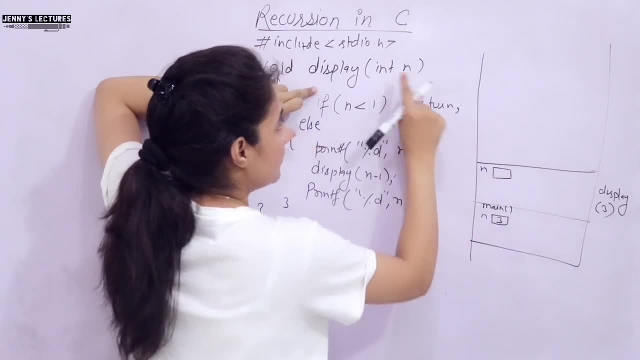 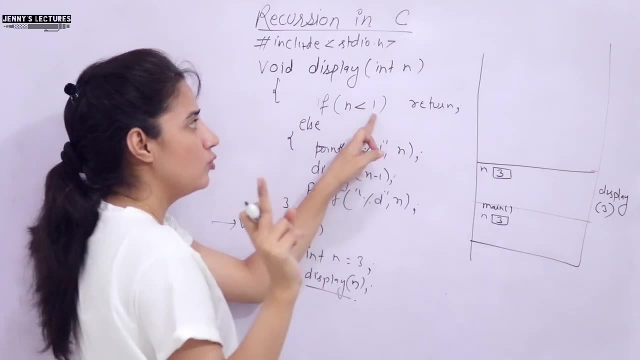 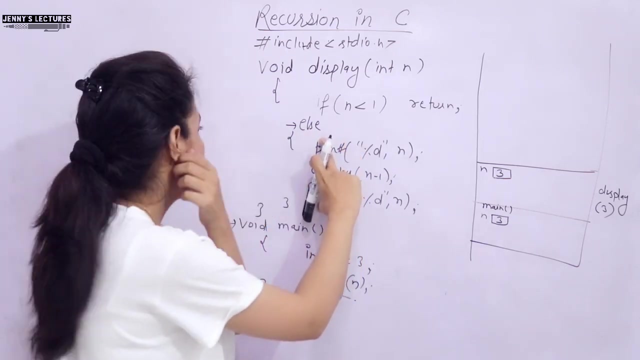 these variables would also be allocated some memory. n is equal to here we have 3, because 3 would be passed. Check the condition: n less than 1. no, this condition is not true. so else part In else part, we have 3 statements. so this thing you have to, you know, check very. 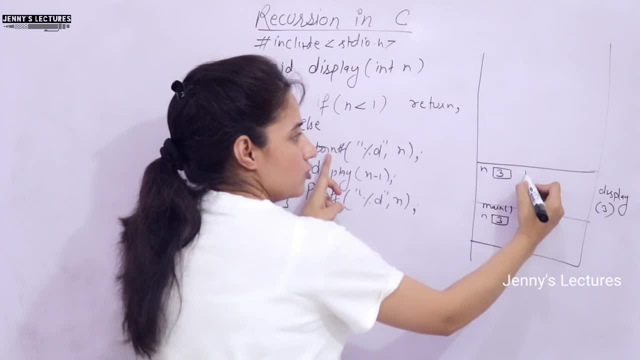 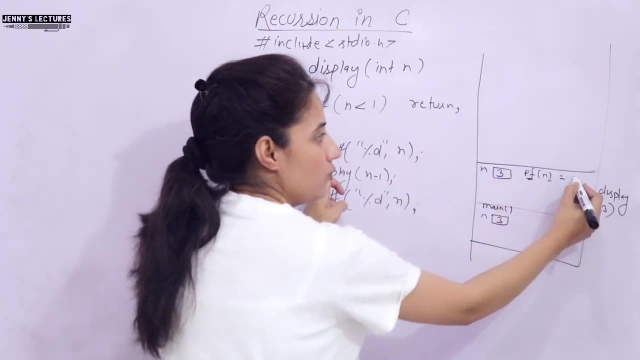 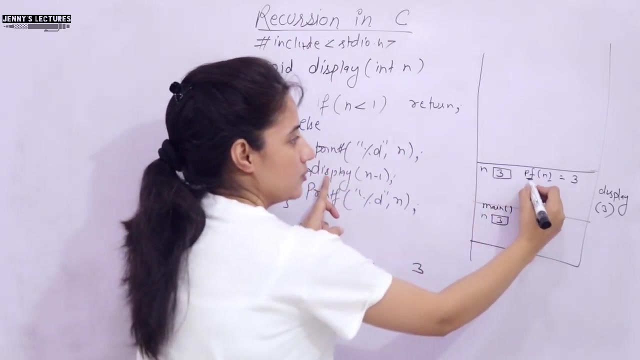 carefully. here we have 3 statements. so first is printf. so first we have printf, so this printf will print what n? so n value here is 3, so it will print 3 on the screen, it will print 3.. Now next statement is display. here we have display n minus 1. n minus 1 means 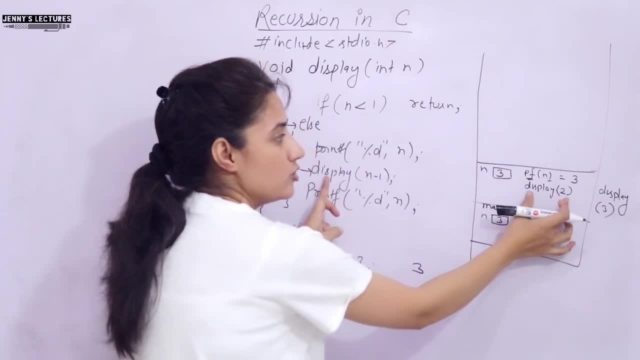 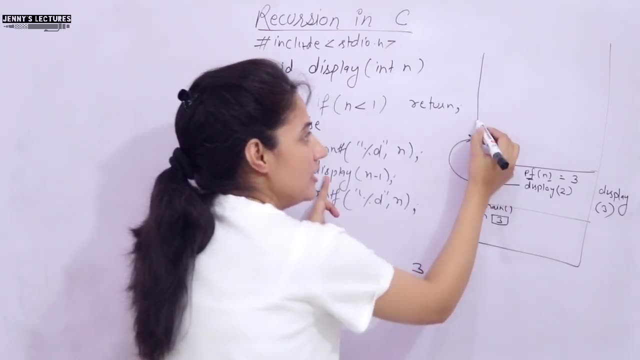 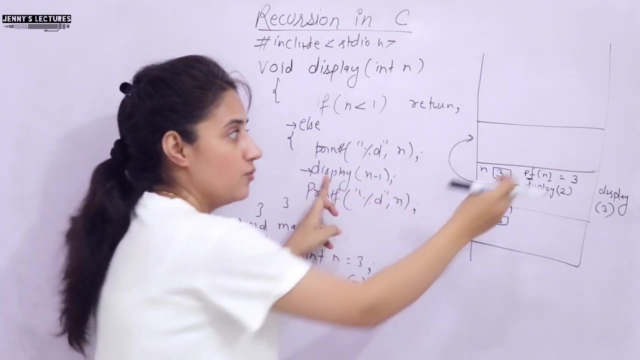 3 minus 1, that is 2. so here we are going to pass 2, and again it is going to call display itself. So when it is going to call itself, obviously above this one, one more frame would be allocated to this function. every time the function would call itself, one frame would be allocated to. 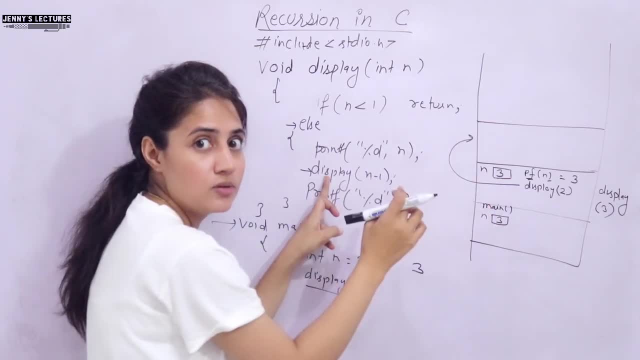 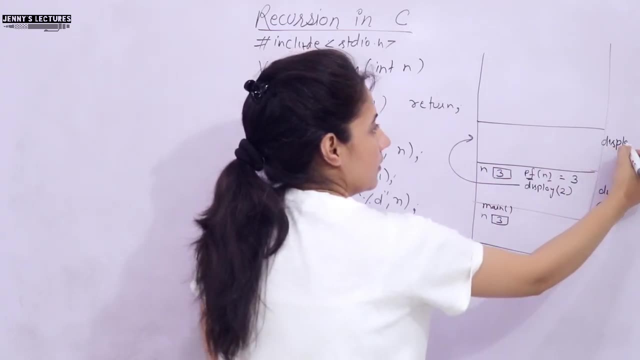 that and these variables, the local variables, the copy of the local variables would be here. So here this display we are calling, but here we have n 2. this is for display 2, right, because from here we are passing 2 n minus 1, 2.. 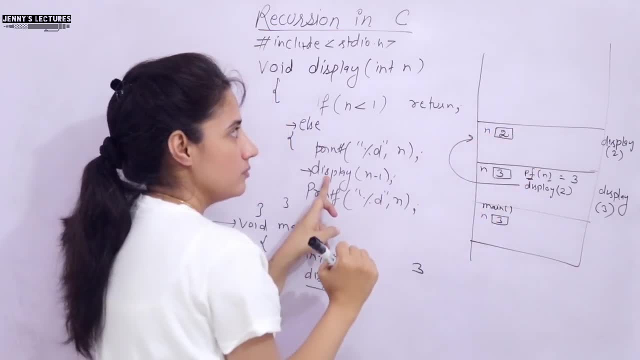 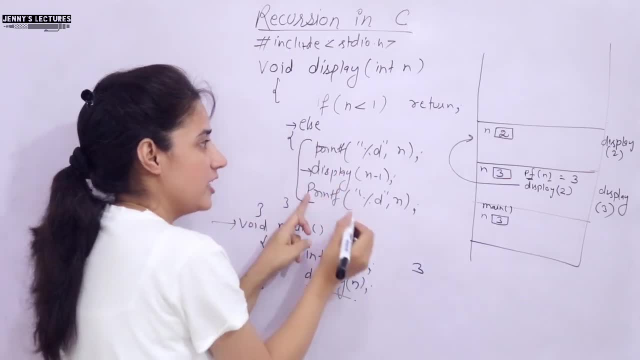 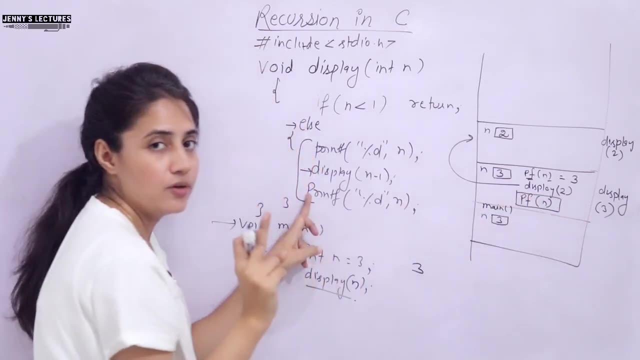 going to into. we are going to enter into else part. in else part again, we have 3 statements: see here. here also we have one more statement, printf n. but this statement is still pending. we have not executed this printf. we have executed this printf only because before this we are. 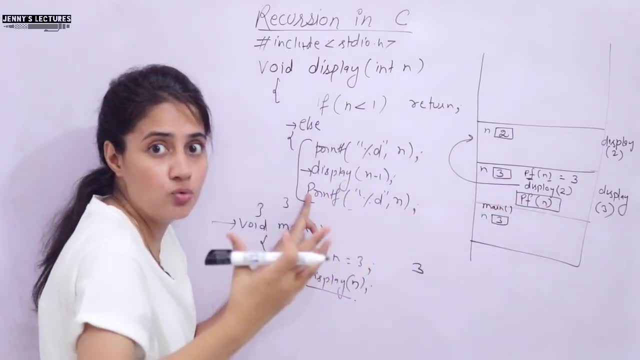 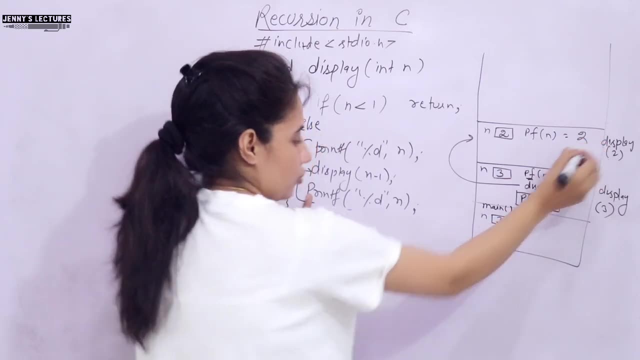 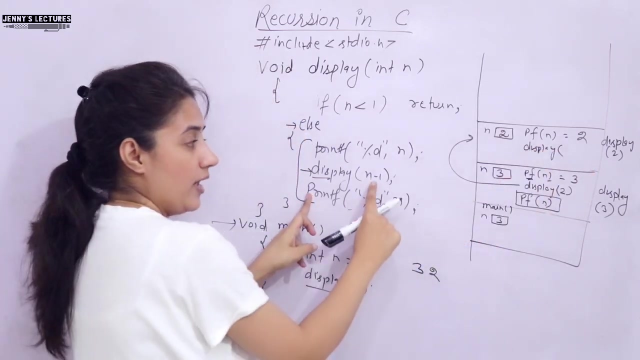 calling this function. so still, this is going to be executed when I will tell you. So now here we are calling display. one printf is there which is printing n, so it will print 2. so in the on the screen it will print 2. now again, next statement is display what we 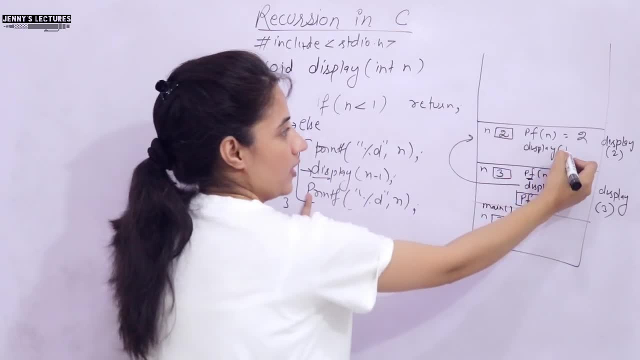 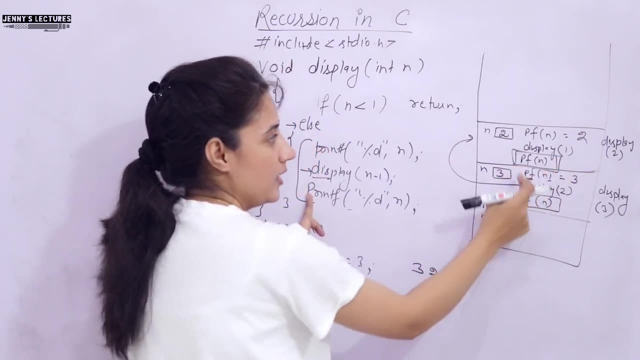 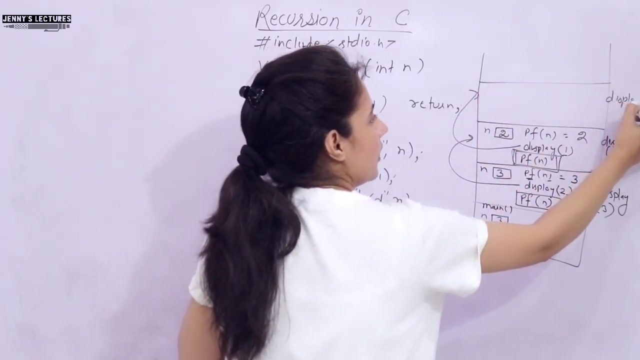 are passing n minus 1. n is 2, so we are passing 1. so, and this printf is still pending, whatever is pending, I am putting that into rectangle. So display 1. so we are going to call the display 1. so again, one frame would be allocated. 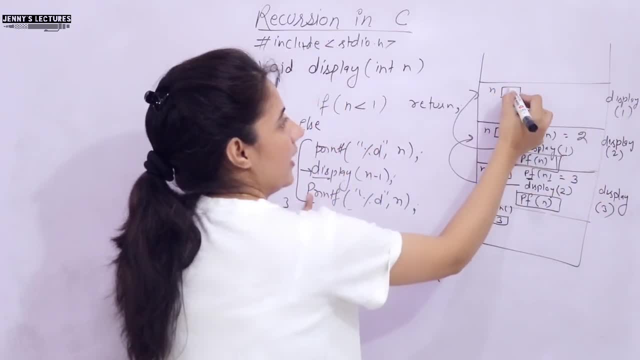 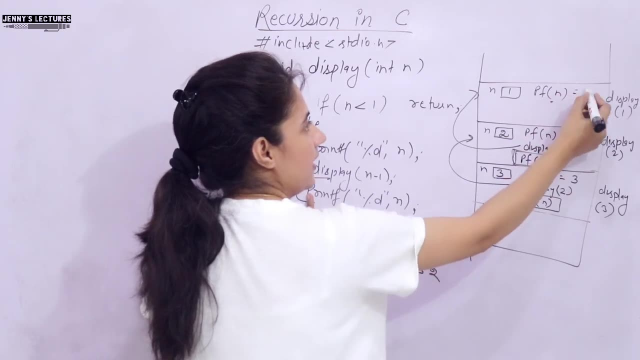 to display 1. this is for display 1. here we have n. n is 1, so less than 1. no, in else part we have 3 statement. one is printf. it will print n, that is 1, so it will print 1 on the. 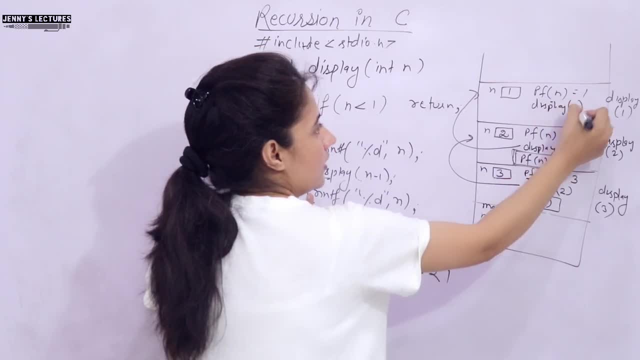 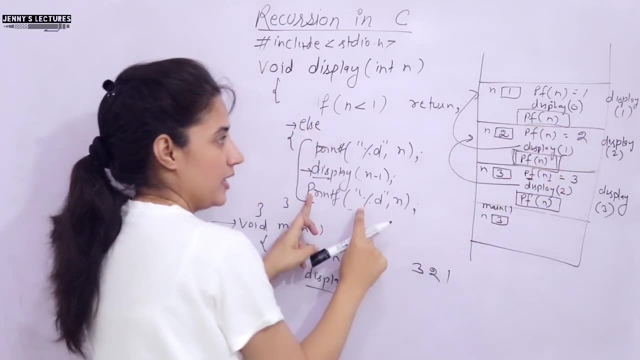 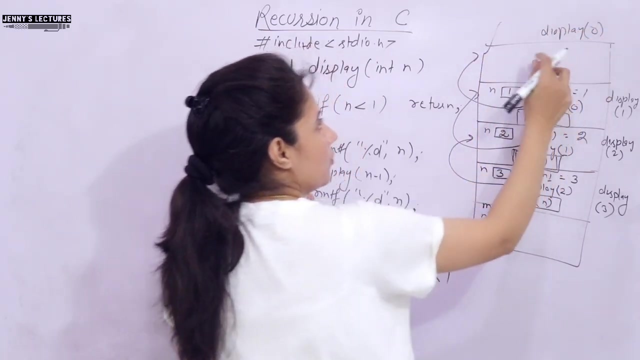 screen again, we will call display display 1 minus 1, that is 0, and here also we have one more printf which is pending this printf. so display 0 means again for display 0, we are passing 0. we have this frame. display 0 would be passed, but this time check the condition. 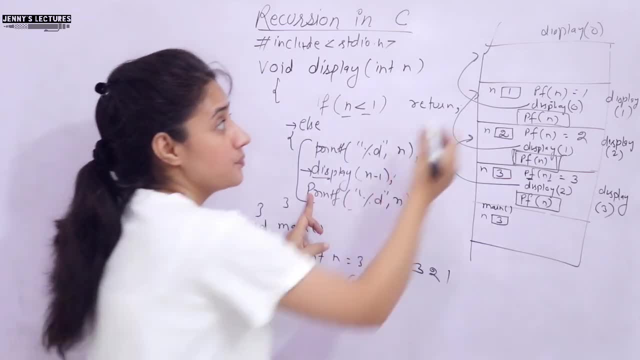 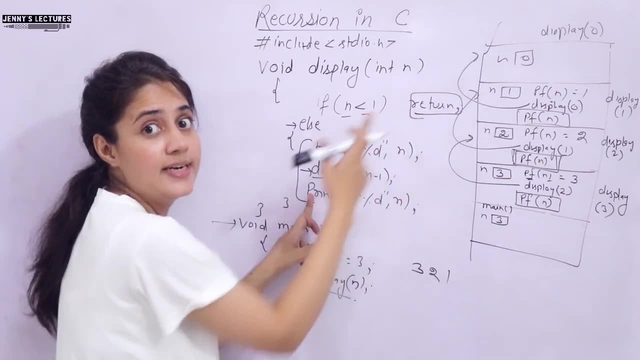 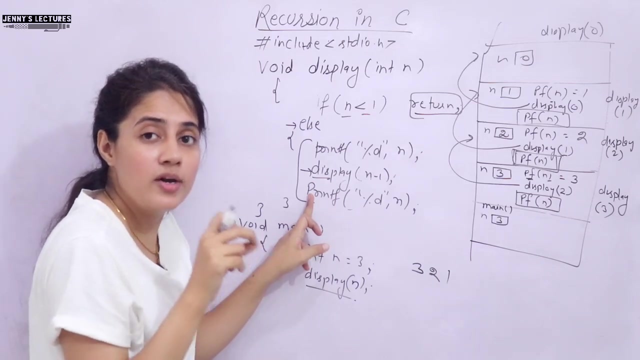 n less than 1 yes condition: true. so here we have n 0. this condition true. now return: we are not going to enter to else part. return is where, simply, this is return. return means where the control will go, the function which are calling this and from where we are calling. 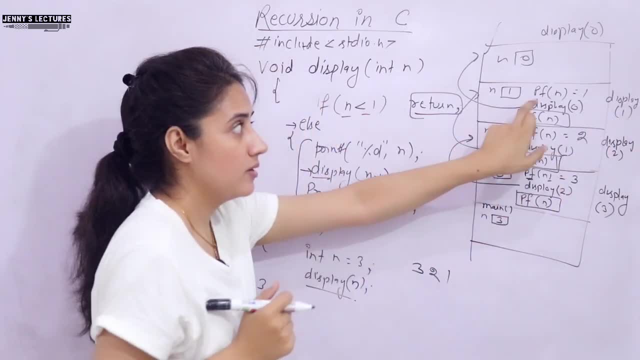 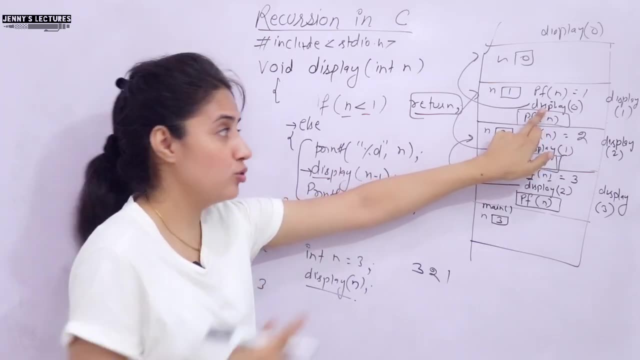 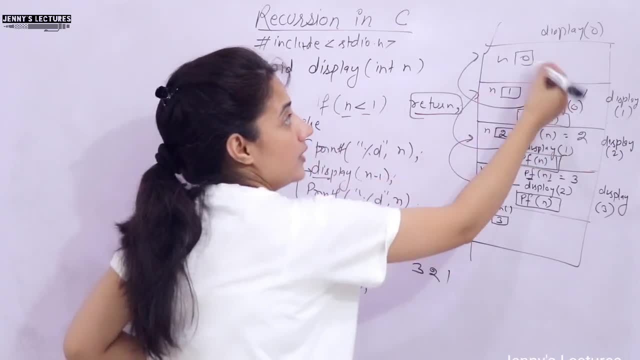 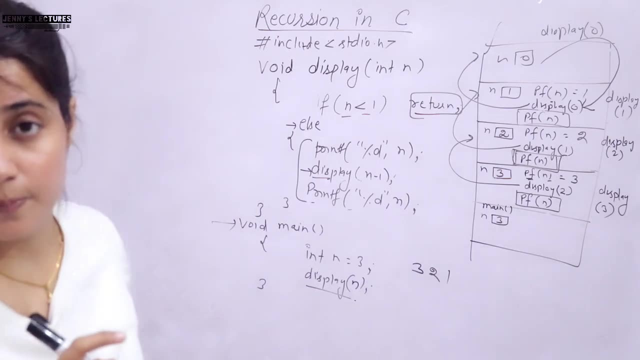 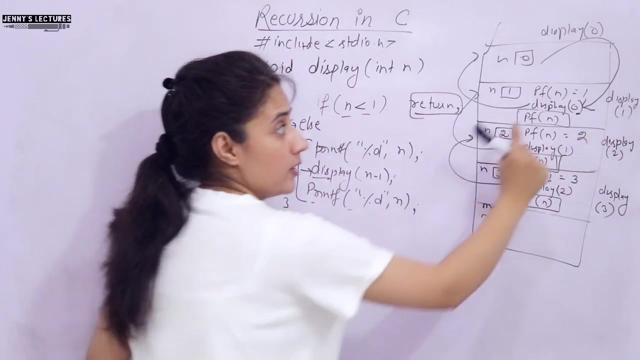 now you have to move backward in the same direction. so now return back. so from here, we are going to return back to here. i hope you can see this. yeah, from here we are going to return back to here. display zero. is there any statement after display zero? yes, we have this statement. 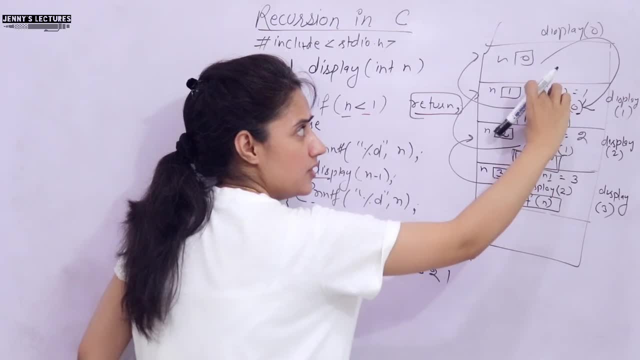 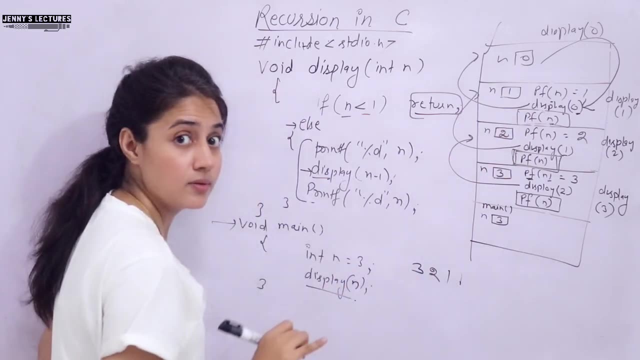 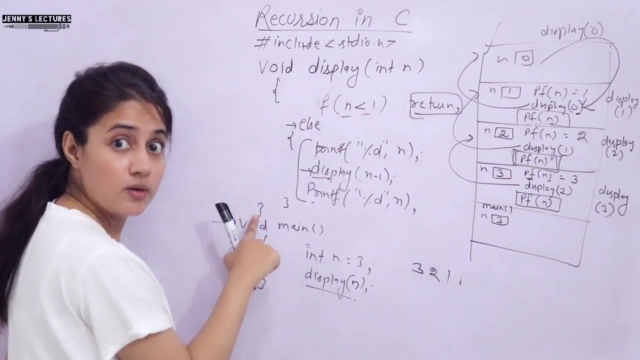 printf n. so what it will print in this, in this stack frame, what is the value of n 1, n, one. so again, it will print one right and after printing, just closing of else, and after this closing of this function, right after closing of this function, obviously the control will return.